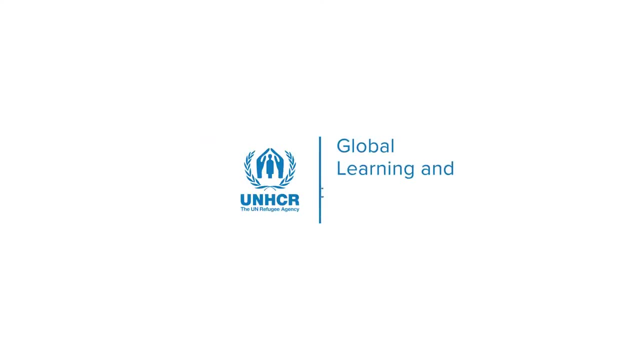 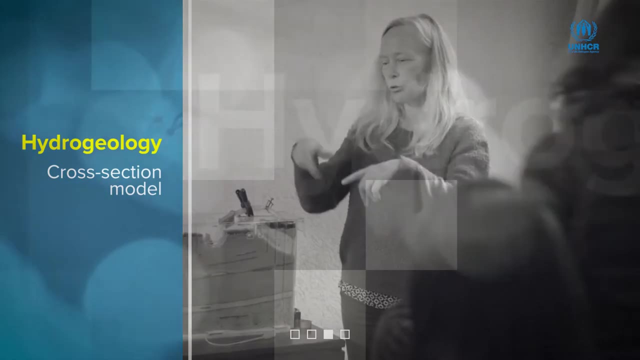 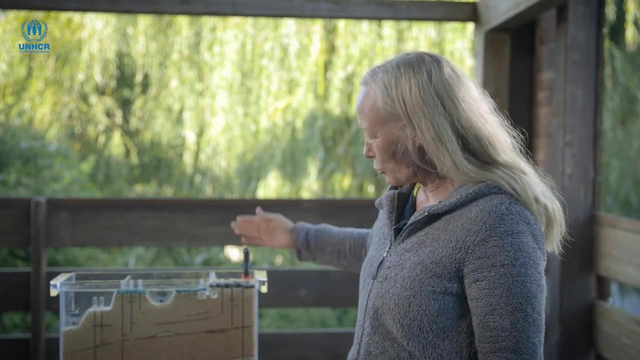 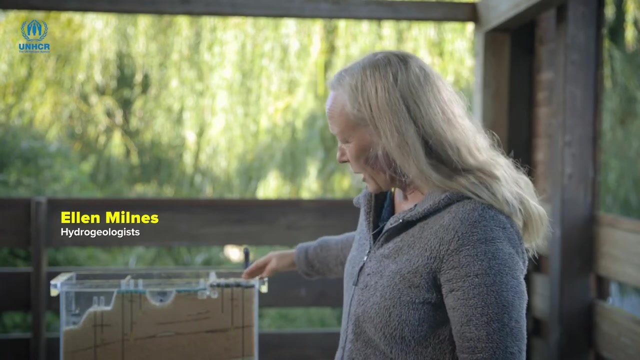 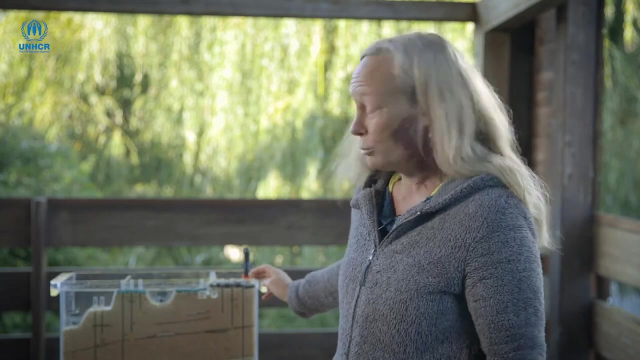 So what we see here is a schematic, small model of a cross-section of a natural area. So what we see here, we could imagine that it is something that covers only a few hundred meters, a few kilometers or even hundreds of kilometers. So, basically, what it allows us to see is the 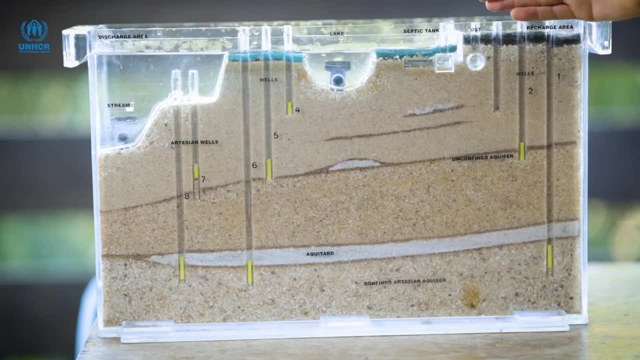 third dimension, the dimension we never see when we are walking here, on the on the surface of the ground. What we see here? a layered aquifer with three different layers with different materials. So all of them are sands. We have a lowest layer here with very coarse sand overlaid. 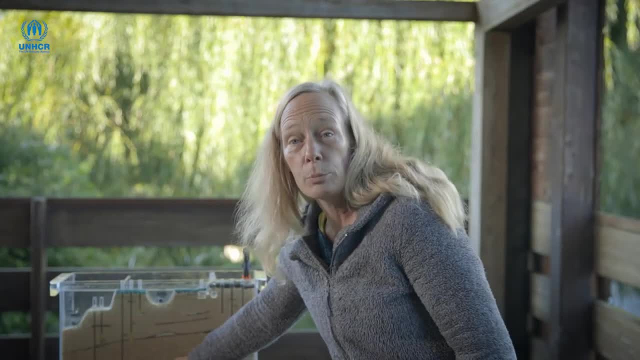 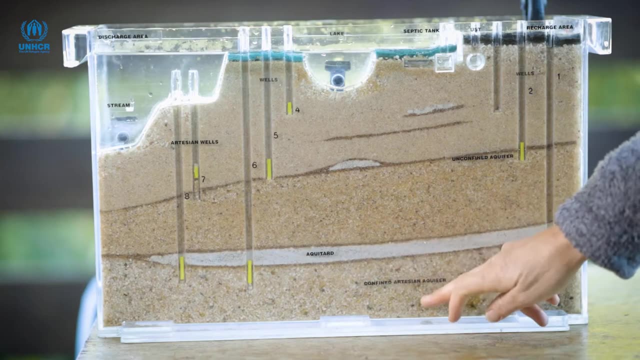 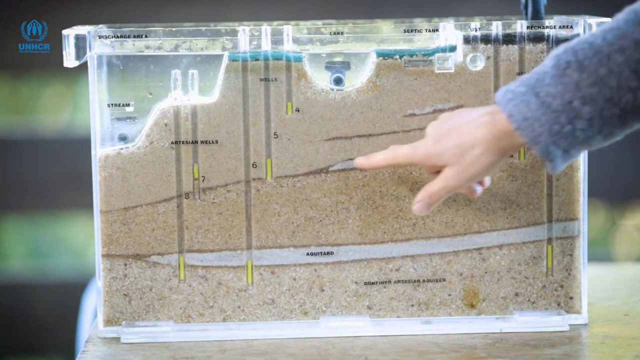 by an impermeable layer that is made up of clay, So it is like a lid on top of this lowest layer, which makes it, which allows it to be pressurized. Now, the top two layers can consist of a medium grain sand and very fine grain sand with some clay lentils in it. Now, what we also see here is that 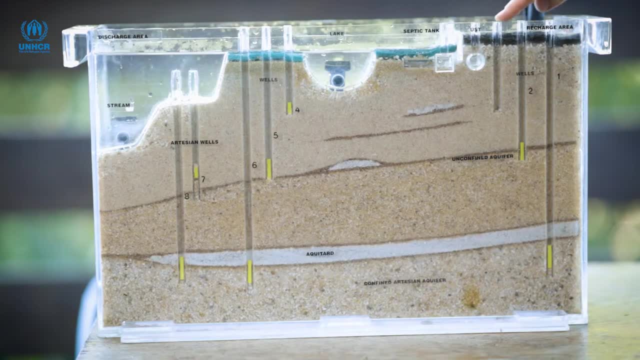 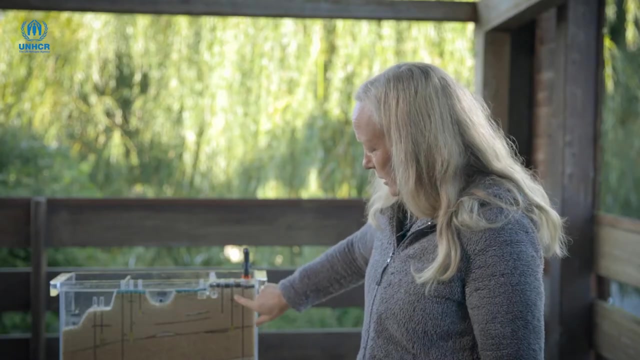 we have a few wells and some infrastructure in this area here that go to different depths, So we have a well that is, we could say almost a shallow well- that is just up in the uppermost layer, and we have a second one going down into the bottom layer And then there is a second layer that is going 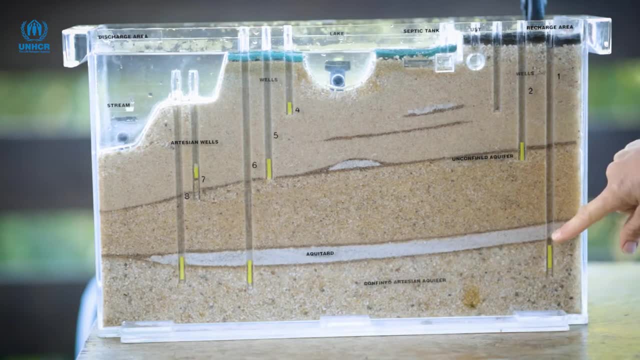 down into the upper layer, and then we have a second one going down into the bottom layer and the second layer and the third one that pierces here this clay layer, to go down to the very bottom, Exactly the same thing you can see here, where we have 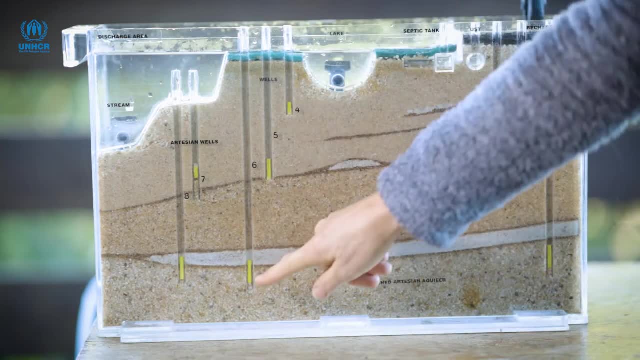 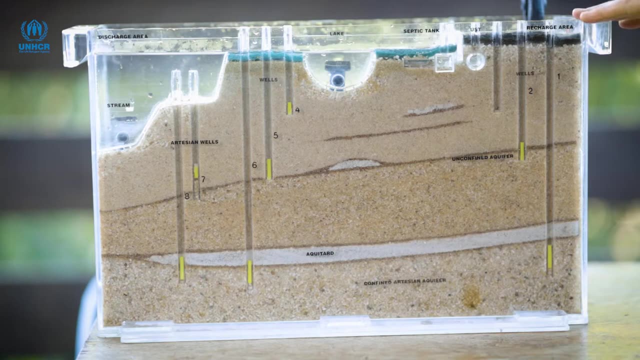 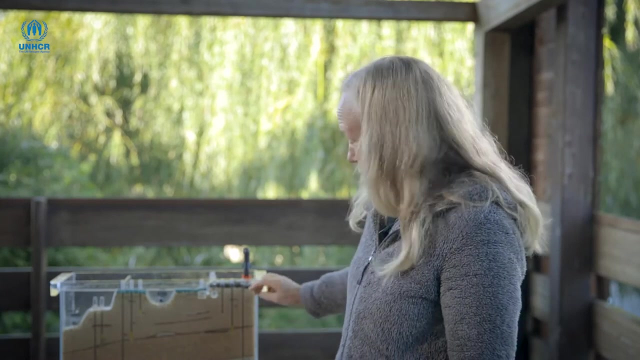 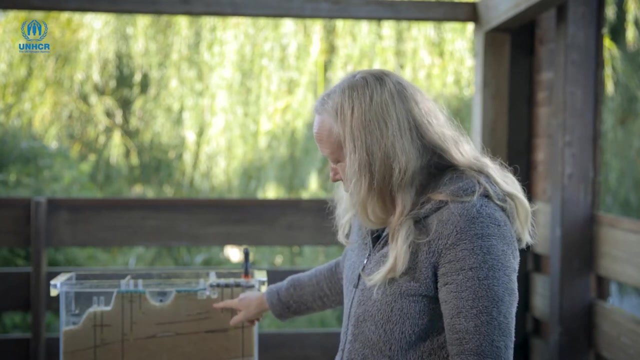 again, three wells going to the different depths and even another one here. So this is now just the description of the material. Now let's look at the water and the water that is contained in all the pore space of all this material. Very often you will have difficulties imagining that there is a lot. 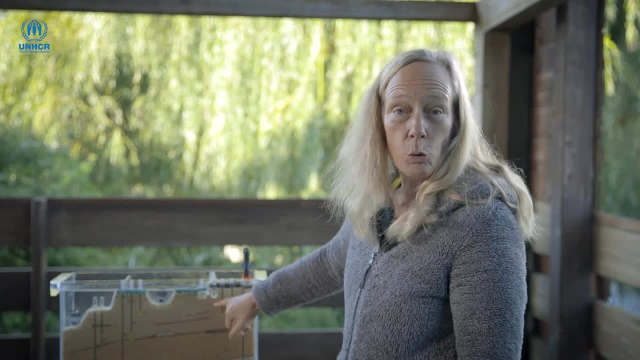 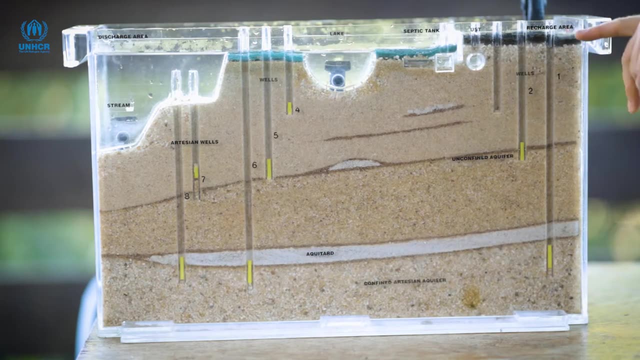 of void here, but actually there may be up to 10 to 20 percent of void space. So there's a lot of water contained in here which you can actually see by the thinking that it is being seriously遊aged up here. So this water kind of 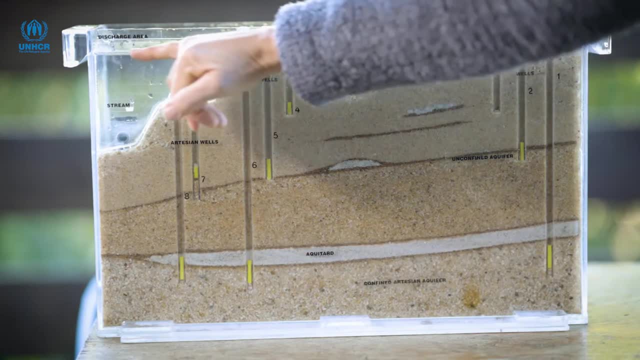 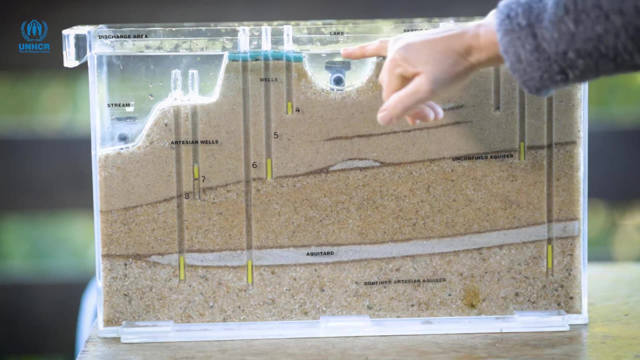 should feel as been in there does and not be touched, so to that This isness doesn't fact that you have. the whole area here is full of water. so in this area here we can see like a lake and the water level goes all the way through and is. 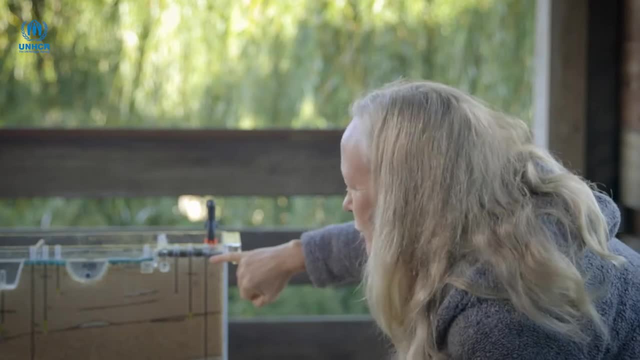 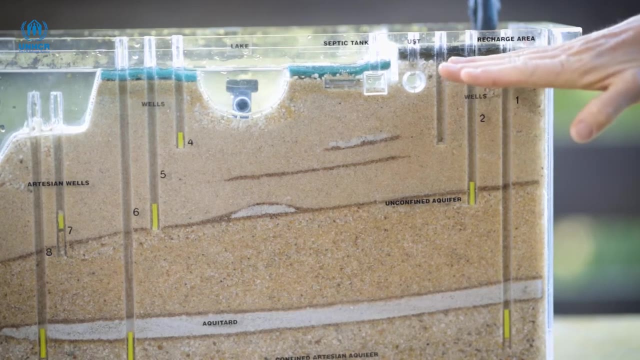 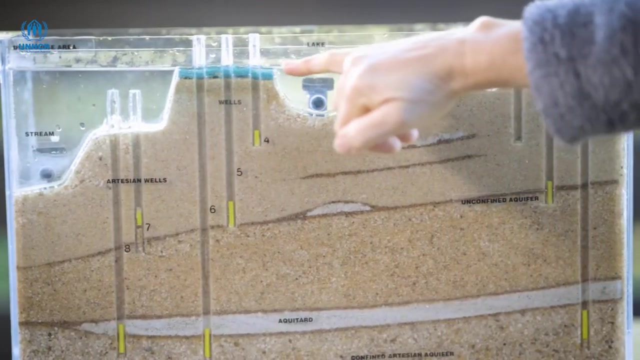 completely stable. It is difficult to see, since it's transparent, but we can actually go and look inside each of the wells and see at which altitude the water level is, and we can measure that everywhere and we will see that it is just a horizontal plane. For water to flow anywhere, we need to get a height. 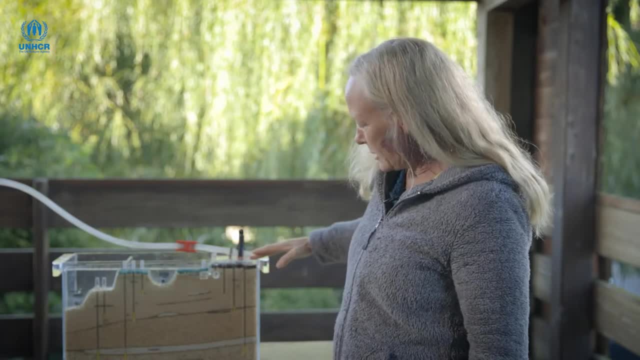 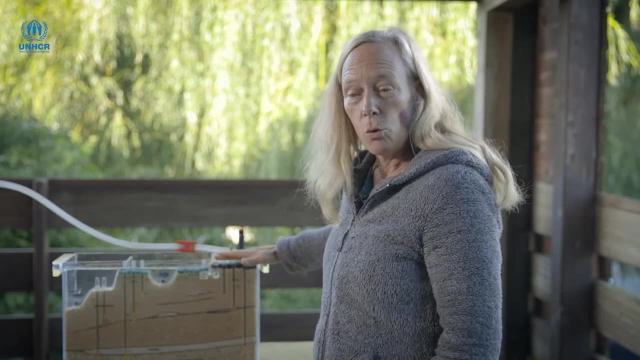 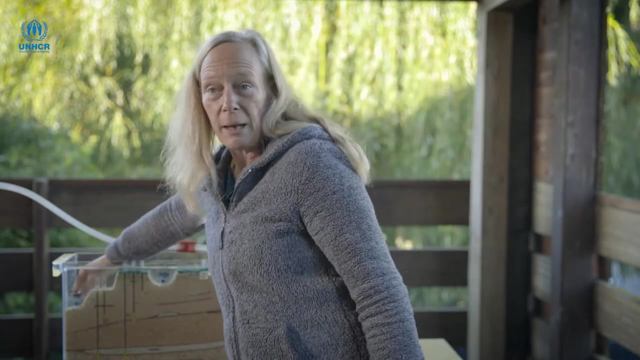 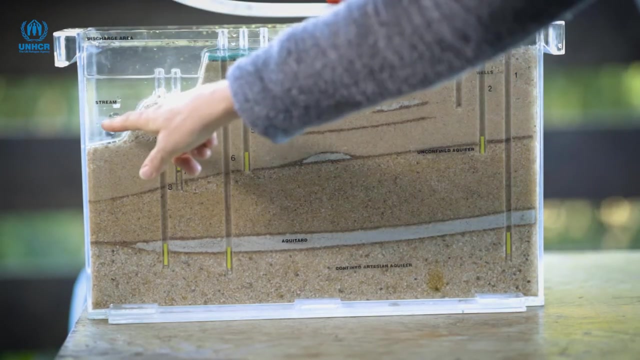 difference. so what happens in nature is that we get areas that are higher up, that are called recharge areas. that is where water infiltrates and feeds the groundwater. but we also need discharge areas. that means places where the water goes out. What we do is we create an outlet, which is here. 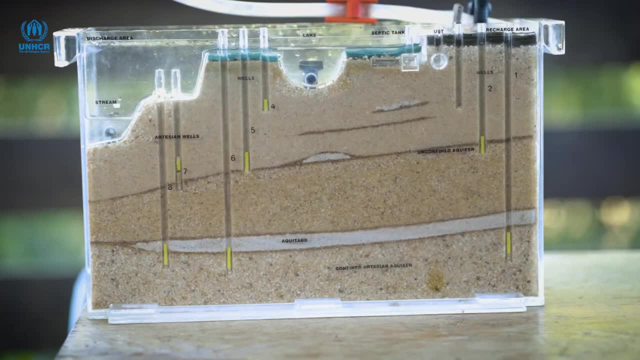 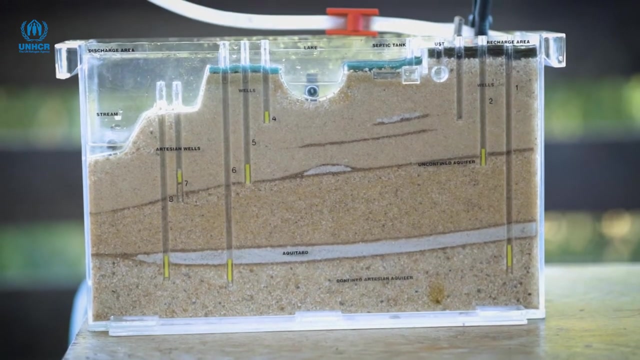 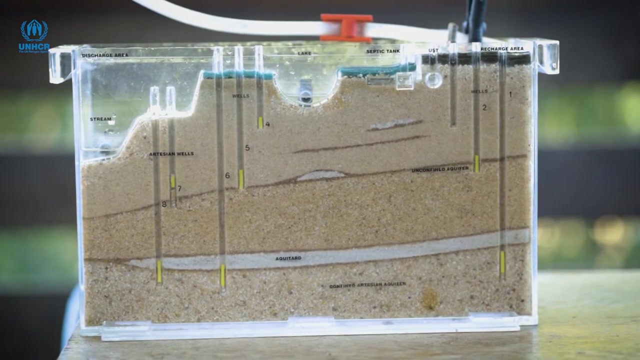 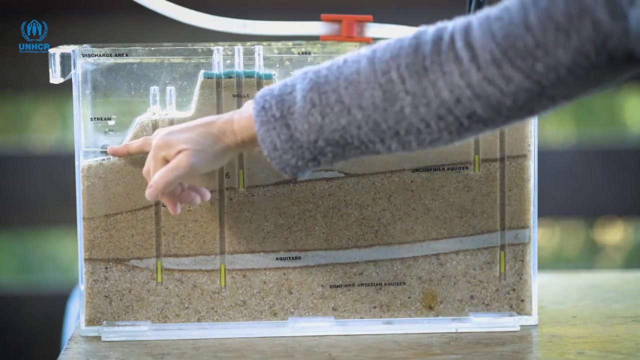 represented by a little stream. So now our area, which was a completely flat here, we have also have a little lake, as you can see. Okay, so what we can see now? before we had one flat water level all along, and now suddenly we have water up here, up here and down here, so it is like a cascading. 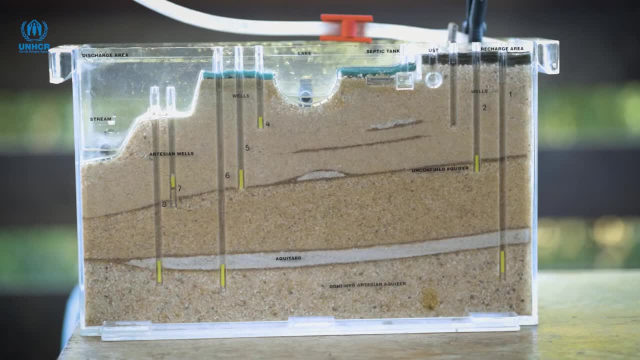 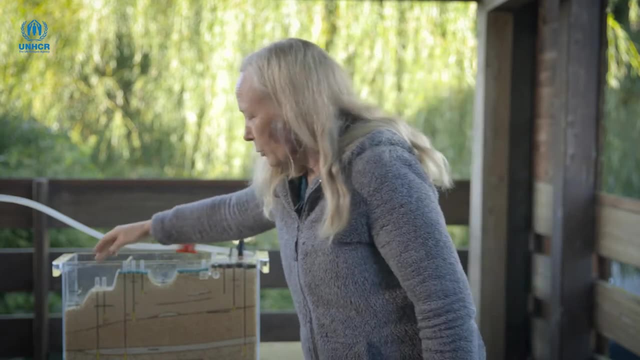 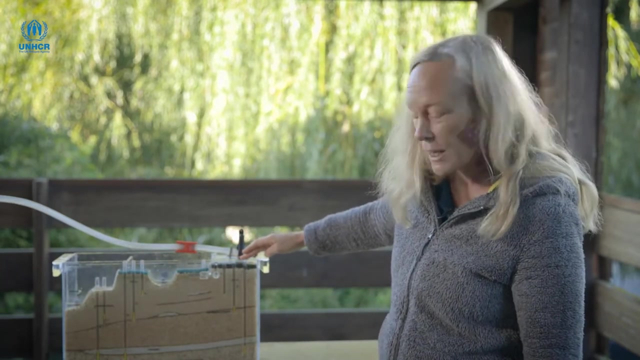 area getting lower and lower down. This is what is required in order for water to be flowing. At the moment, when we look how much water is flowing out on this side, we also know that some water is flowing in on this side, And now this would be interesting to now see what. 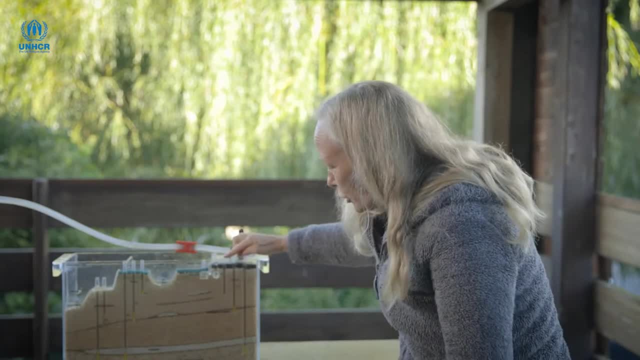 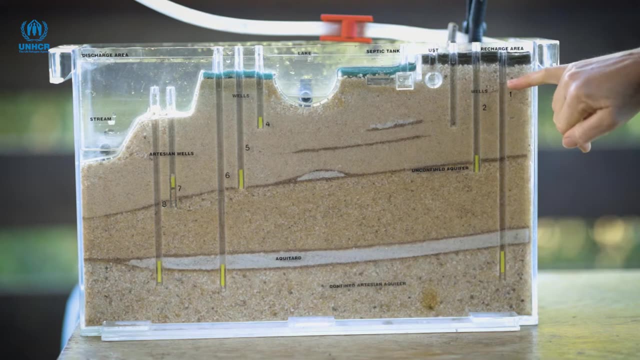 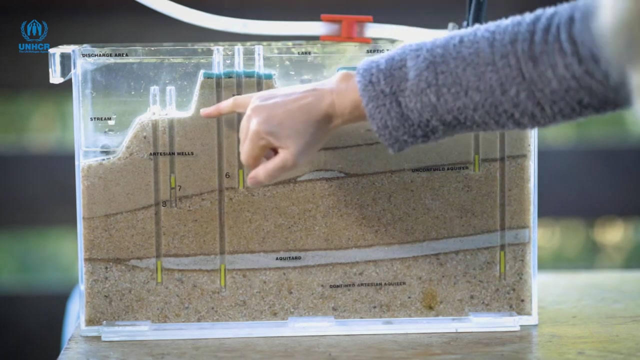 happens with the water levels that we just looked at in these different wells. What you can see in this lowest one is actually a water level that is lower than the one that is just next neighboring, And the third one is even higher up, While in these here we have a high water level here and a water level that is 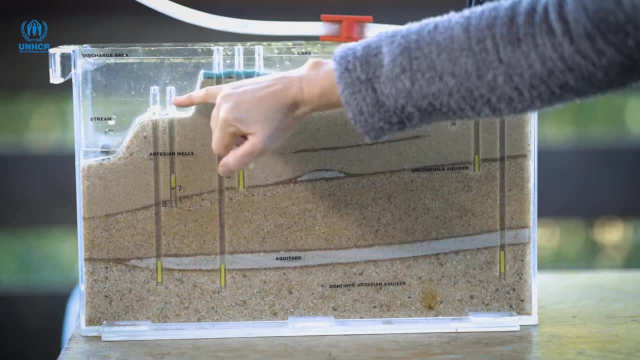 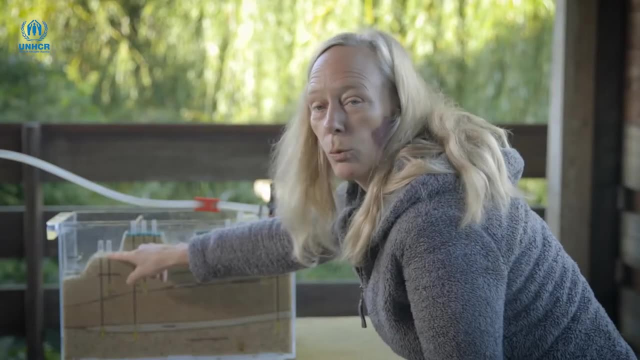 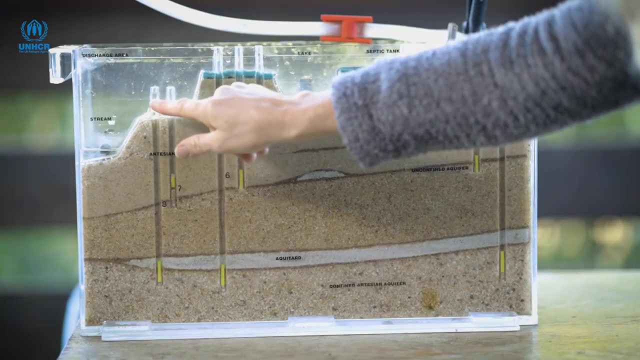 even above the topography in this area here, which is what we call an artesian well, Meaning that if we cut this well, just at the topography, it will be free flowing, it will be just coming out. This means that these this well, here is a. 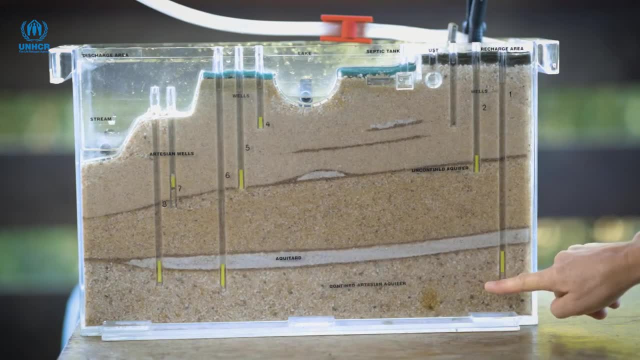 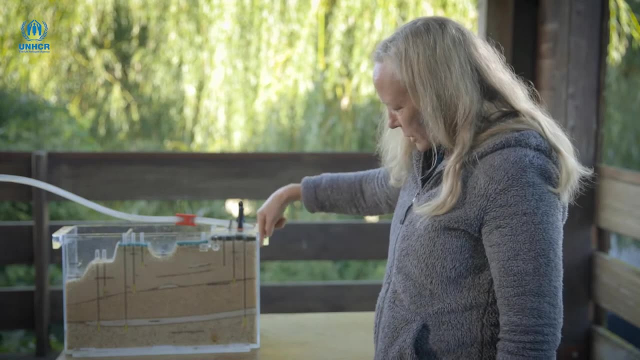 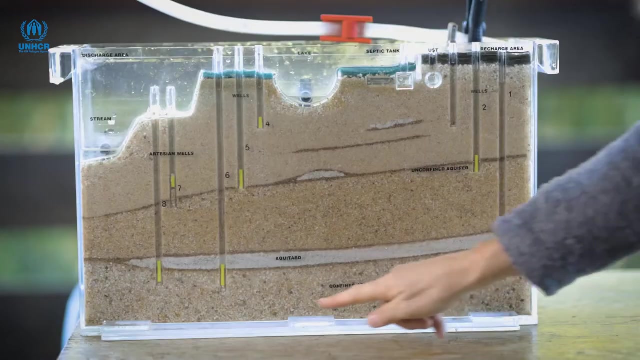 is in a confined layer, meaning pressured layer, This lowest aquifer that we see here. it is actually fed here on the side through a vertical column, so that is where it gets the pressure from, and then the water in here will probably be flowing like this and up there, as we will be seeing afterwards. But how can we? 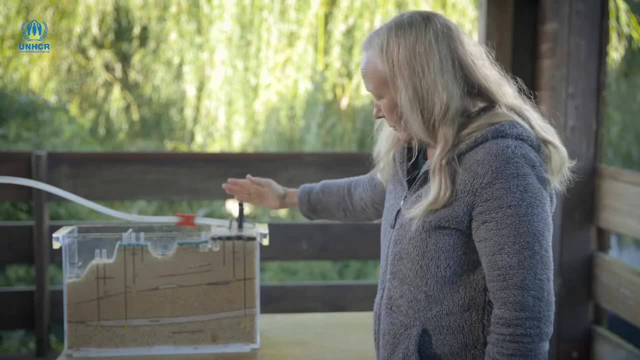 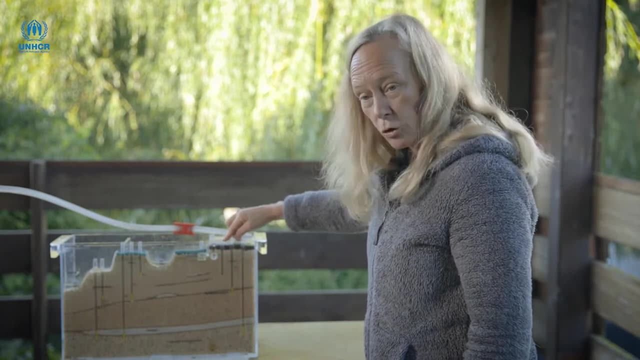 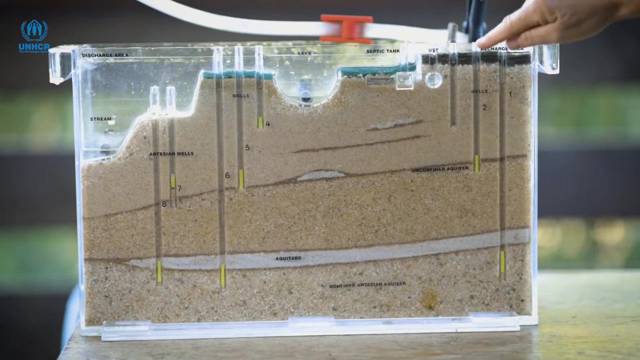 see now how the water flows. This is very difficult in an area like this. We know that they are always flowing according to head differences. So if we look at one aquifer, for instance, the one that is drilled into the second layer here and the second layer here, we can see that the difference in head 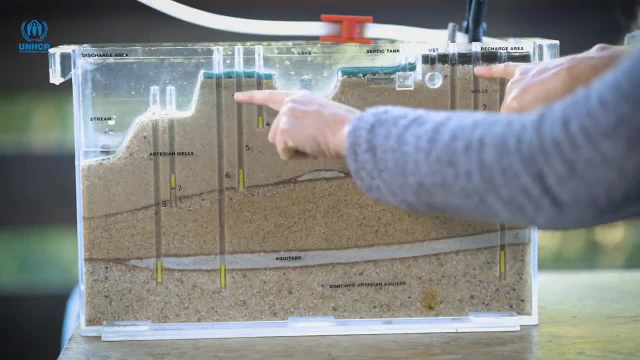 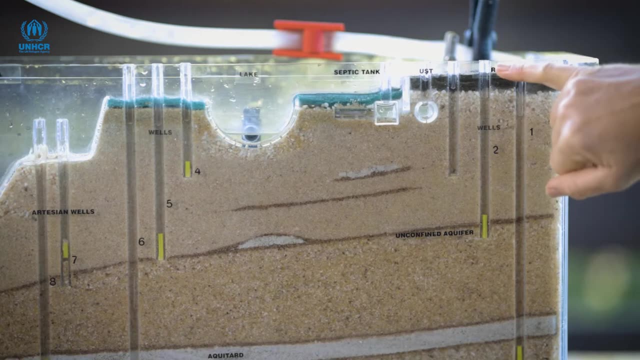 you have one level of height between the head and the DI and you haveidades of height intermediate in head. you have one level of height below health and up here and the other level here which is about one centimeter lower down. You can see in the well number two that is in this aquifer you have the water level. 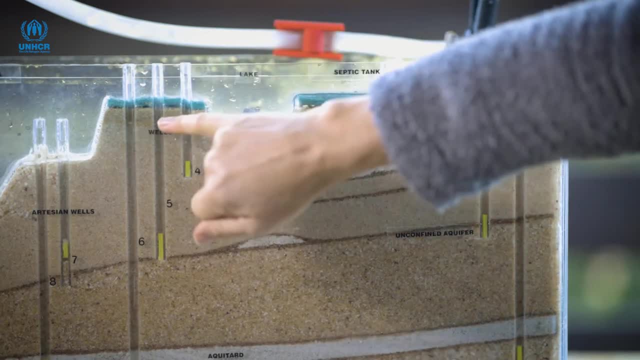 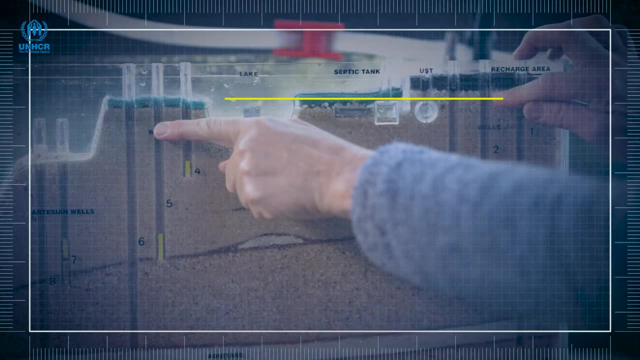 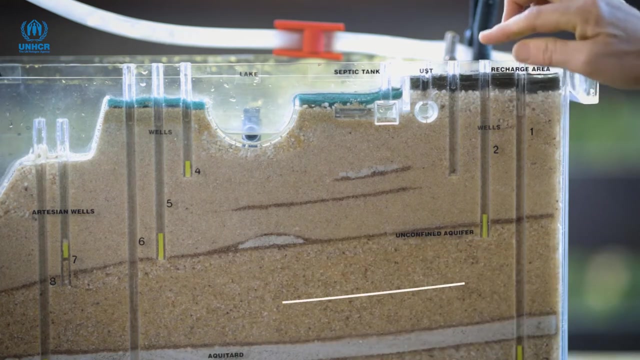 here and in this one. here. you have it there. Now the difference between the two. this is what will drive the water in this direction: from this well to this inside this aquifer layer. Now, the funny thing is you can see in this well, here, the water level is lower than here. 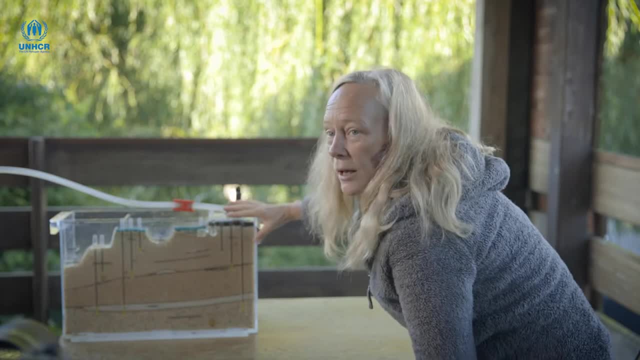 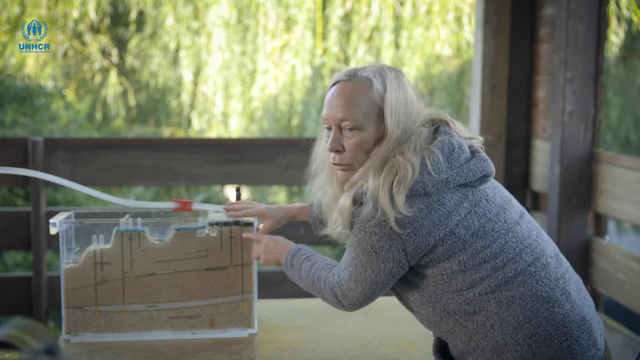 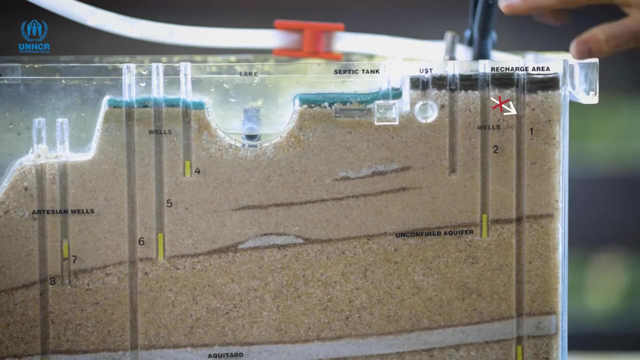 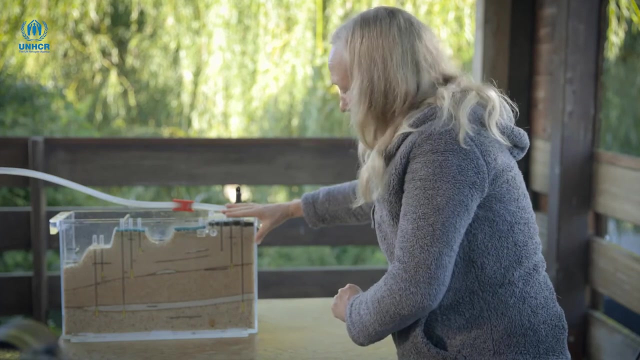 So what you could imagine if you don't know anything about what is happening in this area. but knowing that water is flowing from higher level to lower levels, you would get the impression that the water is flowing from this direction to this direction. So that is why it is extremely important to know the depth at which a well has been drilled. 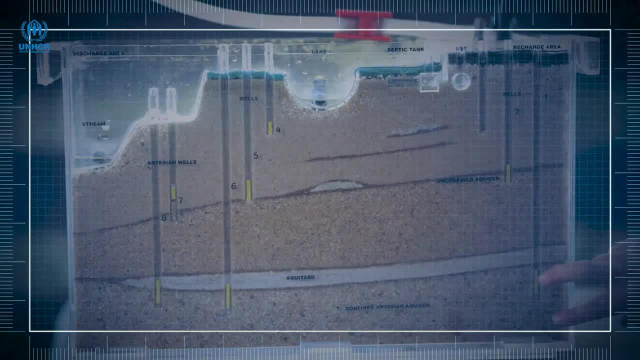 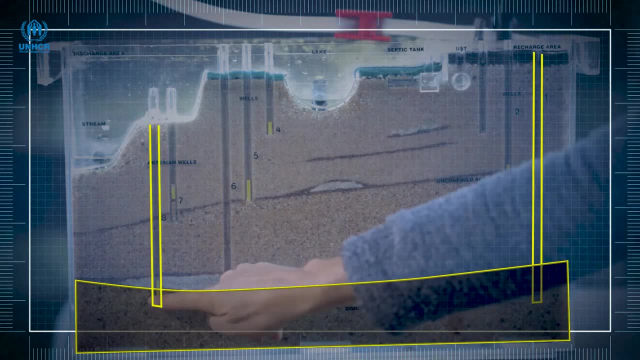 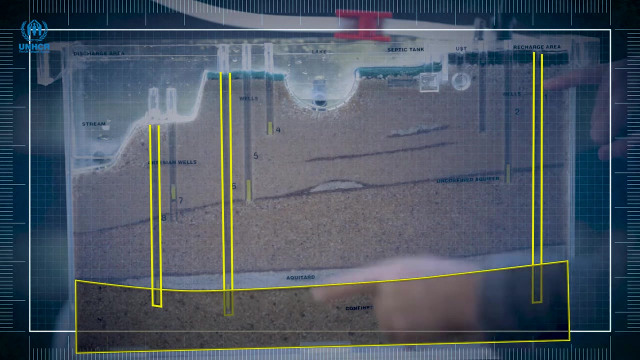 So if we want to know how the water flows in this aquifer layer, we have to compare the water level in this well with the water level in this well or in this well. So here, if we compare number one with number six, we will see that we have again a very 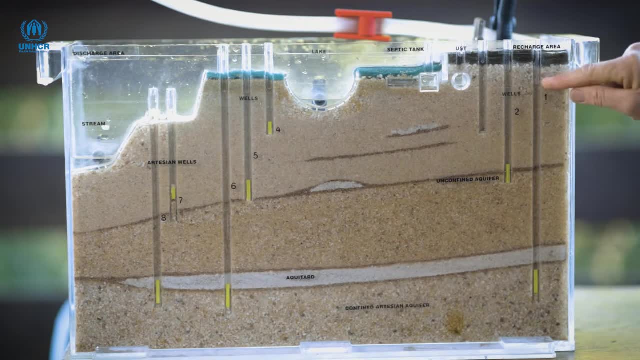 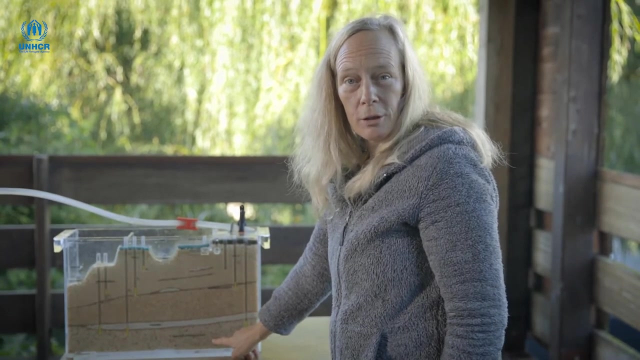 small difference in height. Why is the height difference smaller in this for these two wells rather than for two? These two wells? the reason is that the energy losses in this lower layer are smaller because the material is coarser, So there is less energy that is lost while it is flowing in this direction. 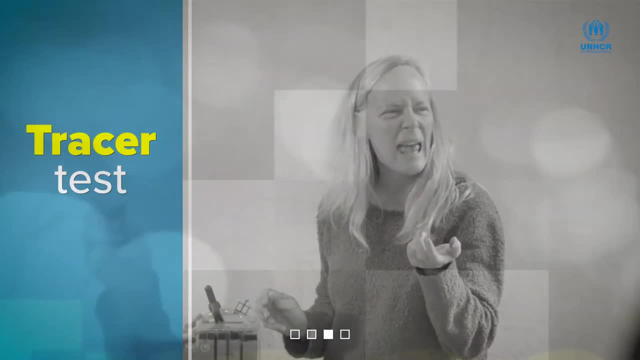 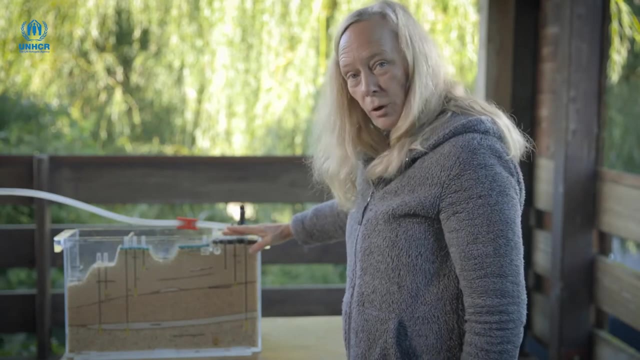 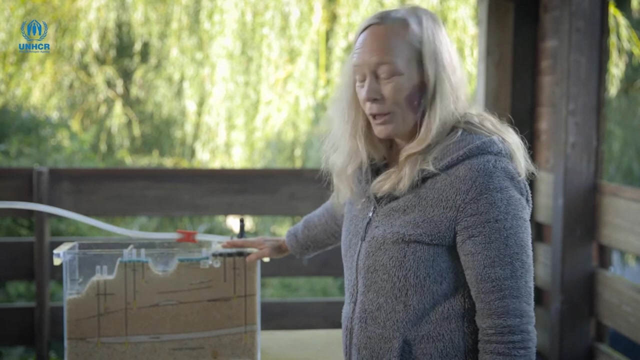 What is the difference between the two wells? To visualize how water is flowing, what we often like to do is to measure the water level. We do something that is called a tracer test, or it is like artificial pollution, which will allow us to really follow these flow lines. 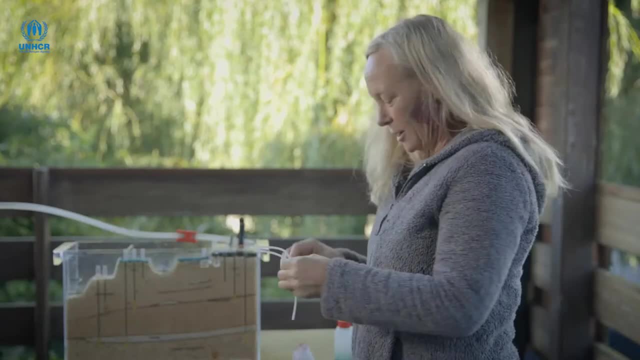 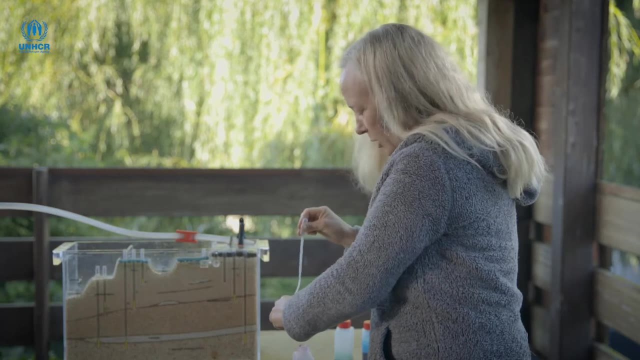 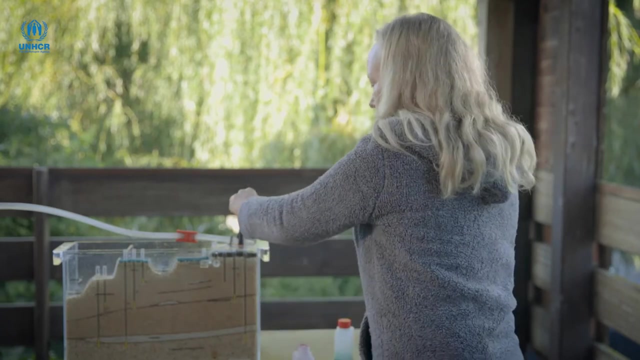 So we will start with the lowest layer. here We will see how it flows, because one thing is just to see the water levels and one thing is to actually trace it and imagine what would happen with any sort of contaminant that would be arriving down in this layer. 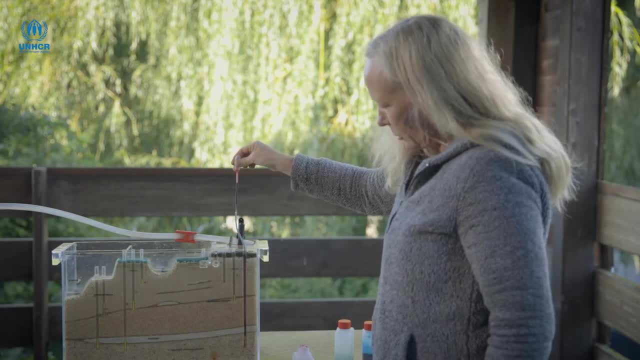 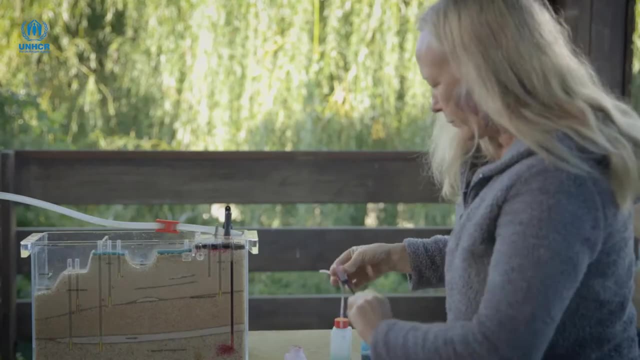 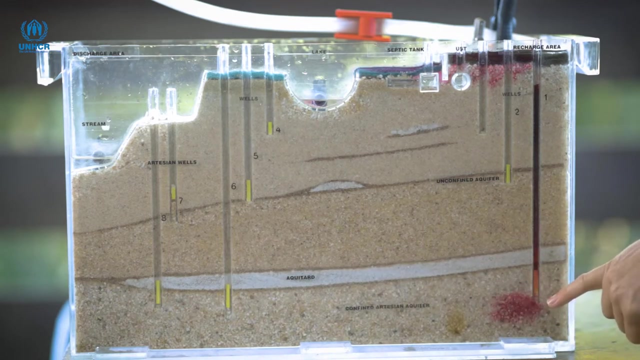 So we just inject a color, So you can immediately see a plume created here at the bottom of this well, which is due to the fact that I was injecting a contaminant or a color in this area, and you see it immediately starting to flow in this direction. 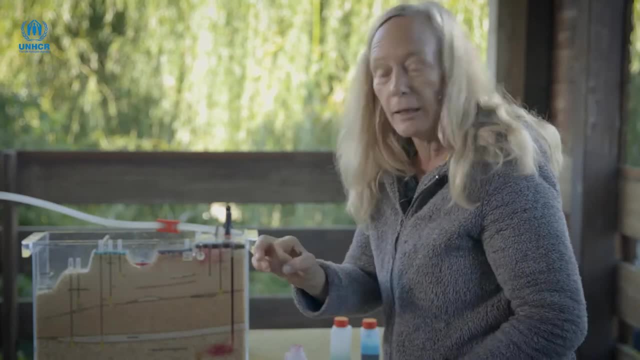 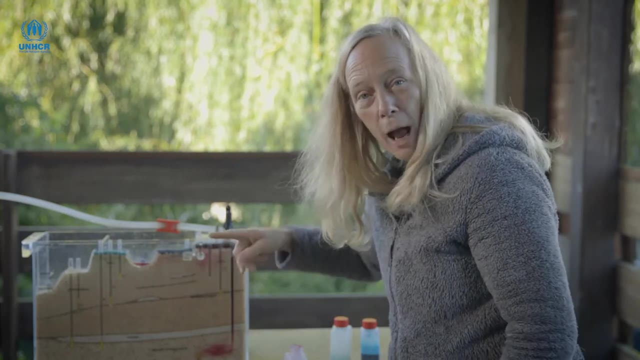 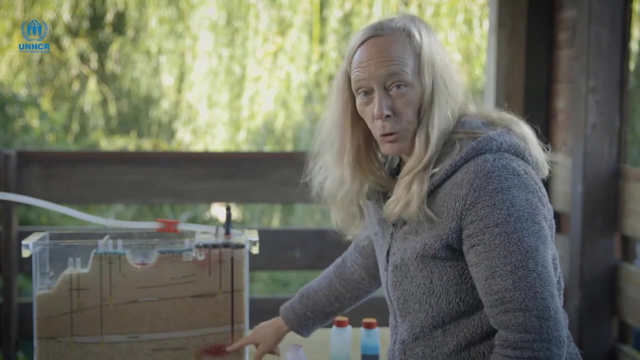 So now, why doesn't it just stay together like a little spot? Why does it get bigger? Well, it is that actually, all the pathways around these grains- there are multiple pathways that have different lengths, So this is what we call dispersion. 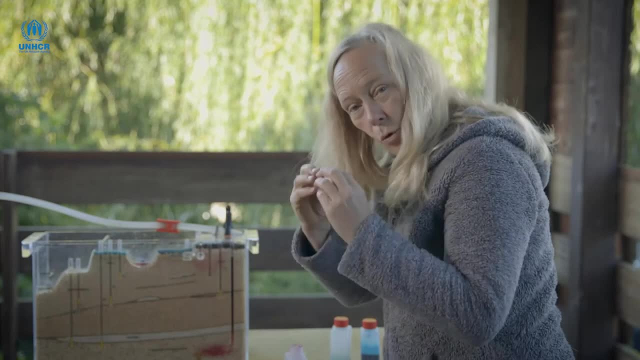 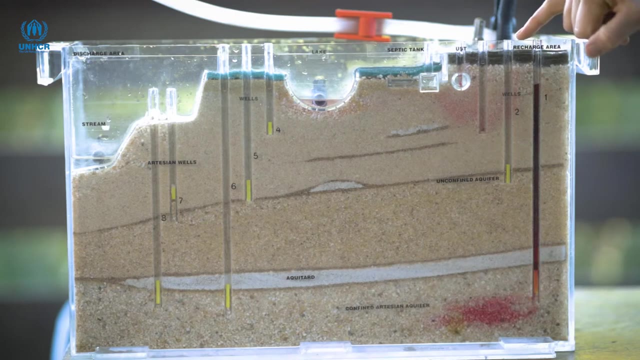 So the faster this whole plume goes, the more this this plume will be elongated. At the same time, you could also see that some of the contaminant actually infiltrated here at the top, which is already contaminating this upper part. 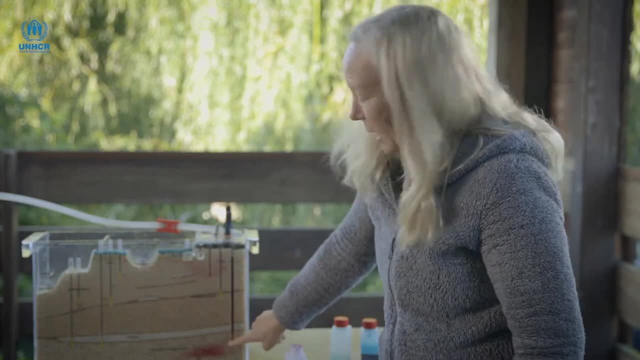 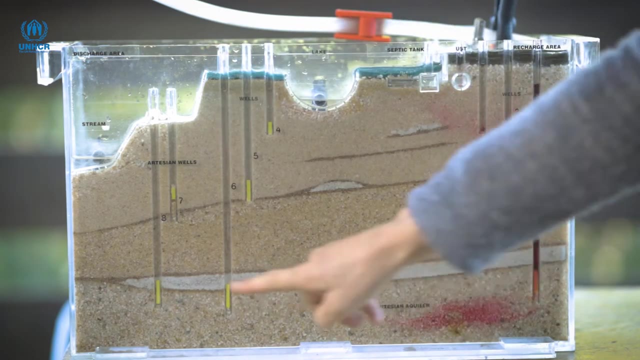 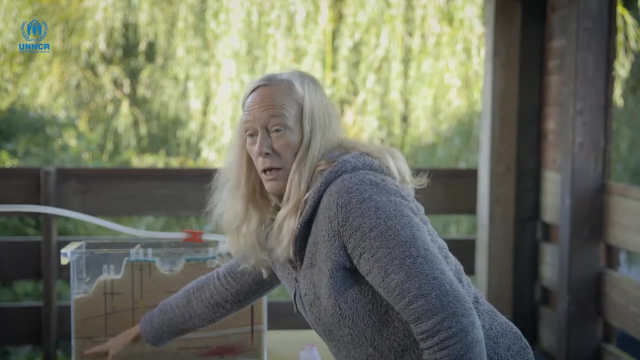 So where would we expect this contaminant now to arrive? It is very likely that we will be seeing it appear in this well, but also in this well. And then where would it arrive at the very end? Will it stay down here? 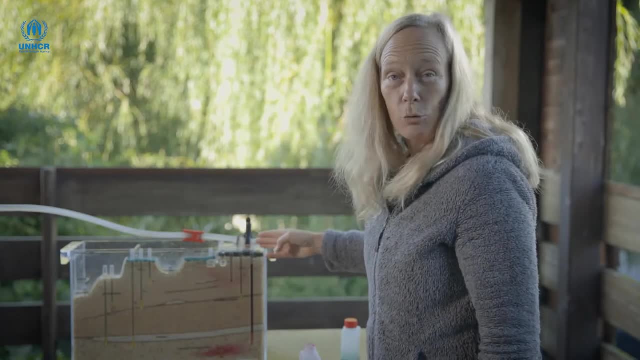 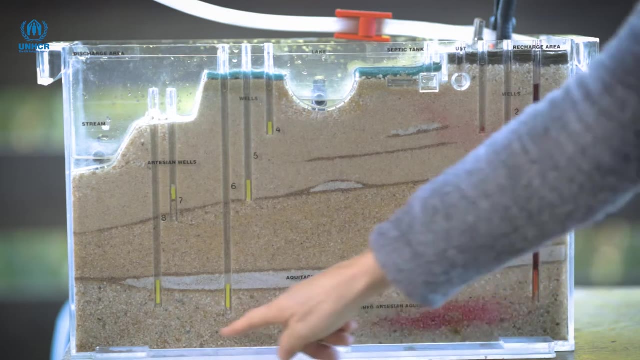 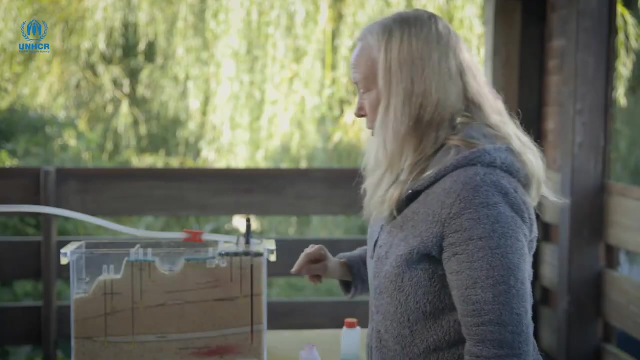 No, There is just one way that the water can go from an input to an output. It means if water is flowing here, there is only one place it can come out, So eventually it will have to flow upwards towards this stream. 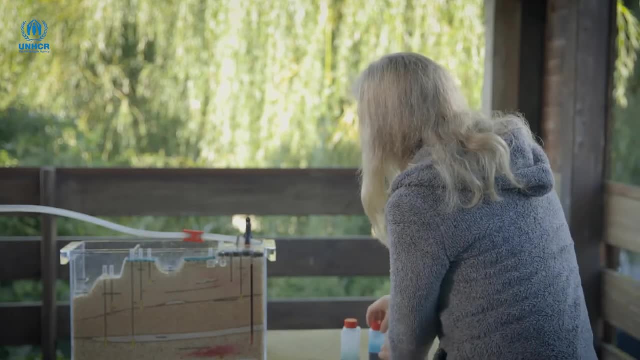 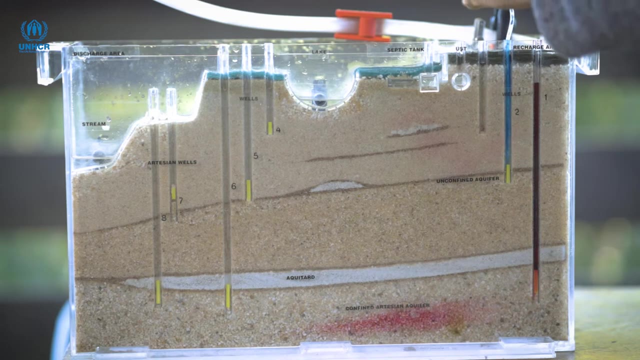 So let's do the same exercise with the second. well, I'll take a blue one for this one. I'll try to do it very quickly, Very nicely. You can see a very dense plume developing just at the bottom of this. well, 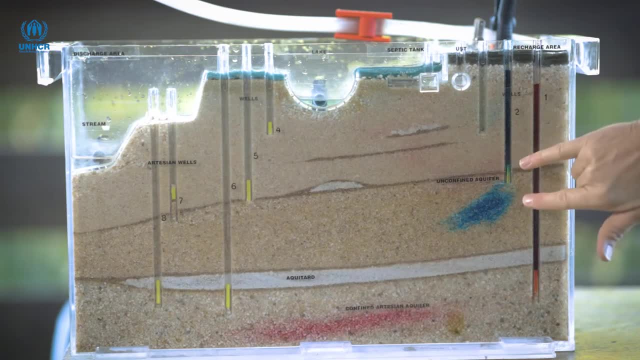 So you can see here now that this plume actually doesn't go straight like this. It doesn't go straight like that. It is actually going in this direction. So it means that flow Flow is always perpendicular to the piezometric lines. 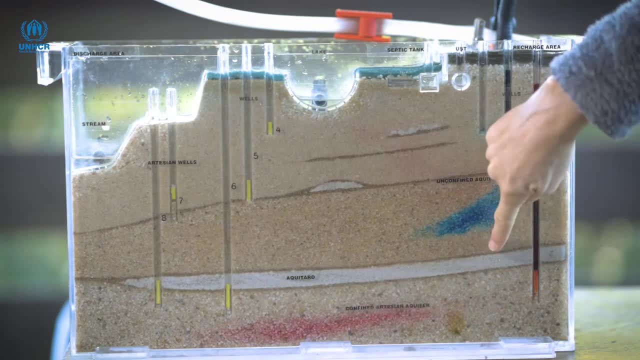 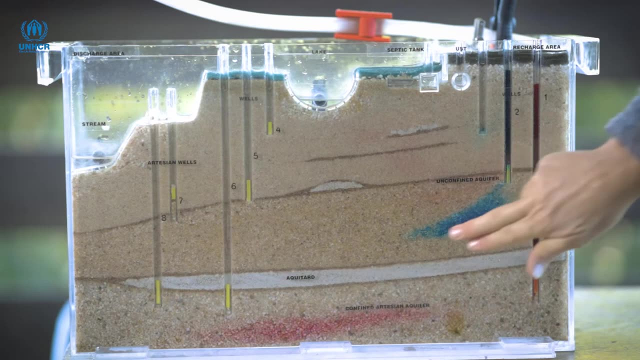 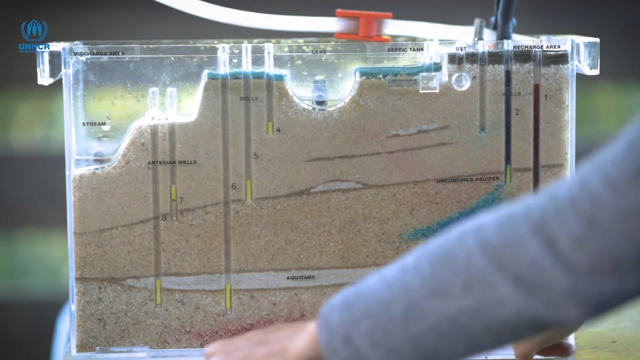 It means that if we had to draw now the piezometric lines, they would have to be somehow like this in order to be perpendicular to the flow lines At the same time. now you can see at the bottom how wide this red plume has become. 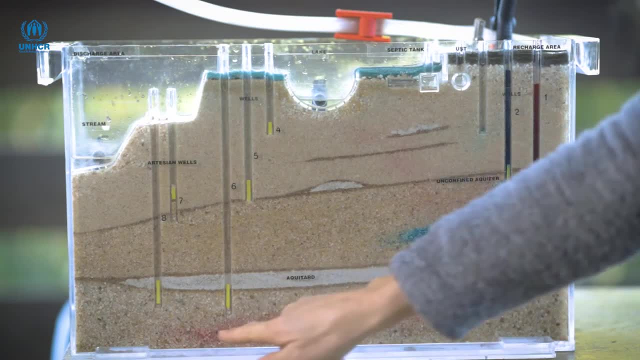 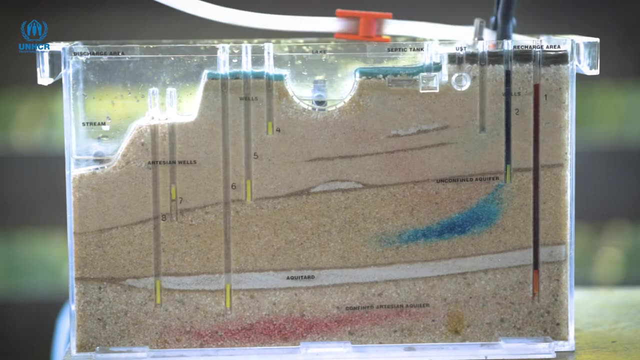 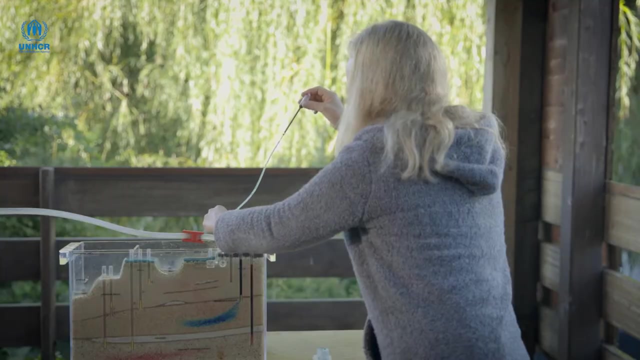 It has become. There are some very slow ones here, some very fast ones here, and some of them have already reached this well. So if we now pump in this, well, you will see that some of it will come up, But before we do that, we will even contaminate the third, which is the most shallow one. 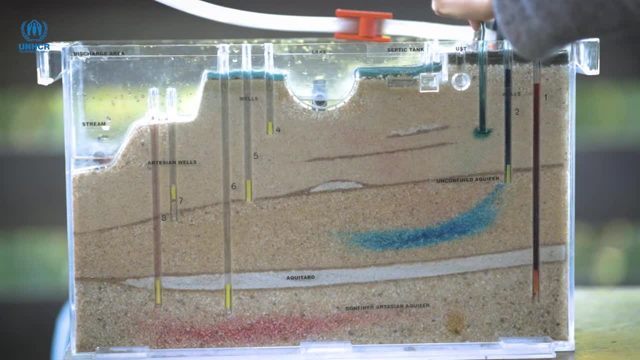 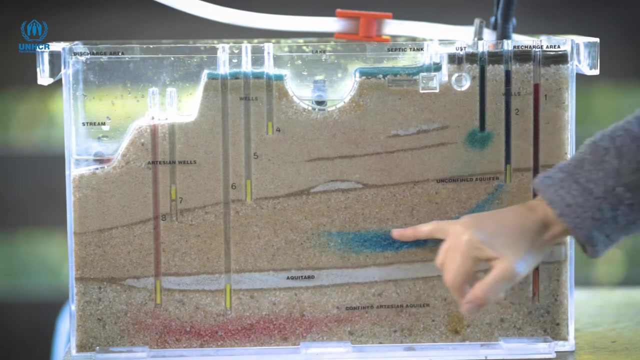 Let's see Now. that's a very intensive one, So definitely in this area. here we have like almost horizontal flow in this direction, because the plume is obviously following, staying inside this medium-grained sand. Now it will be interesting to see. 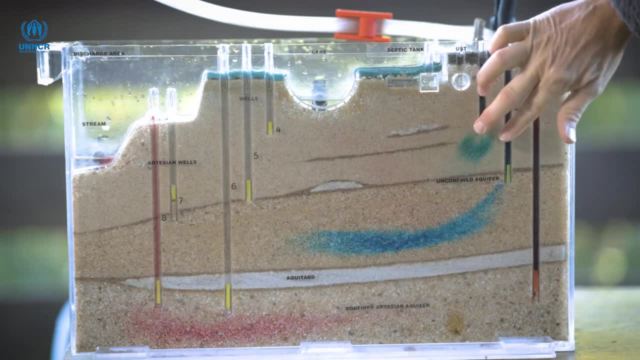 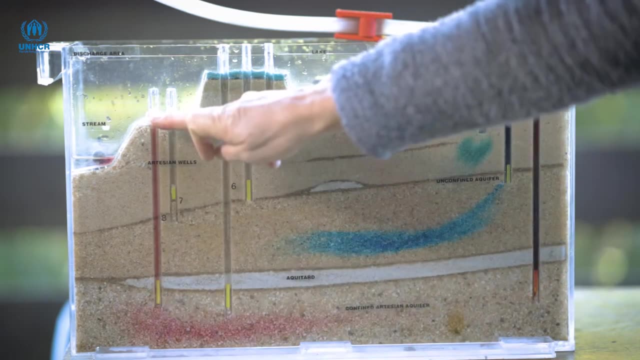 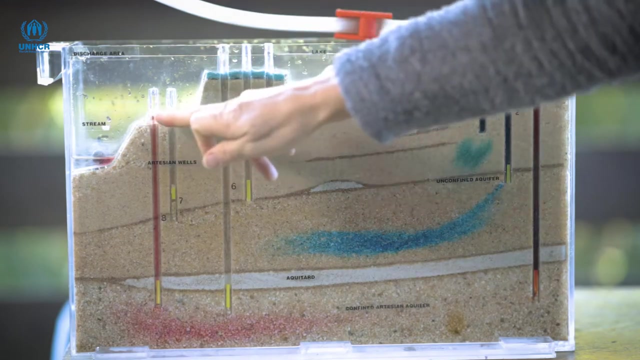 As you see where this one goes, it obviously has a downward direction at the moment, while the red one at the bottom you can see it has already, in the meantime, contaminated one of the wells. Now this is a very interesting thing that can happen. 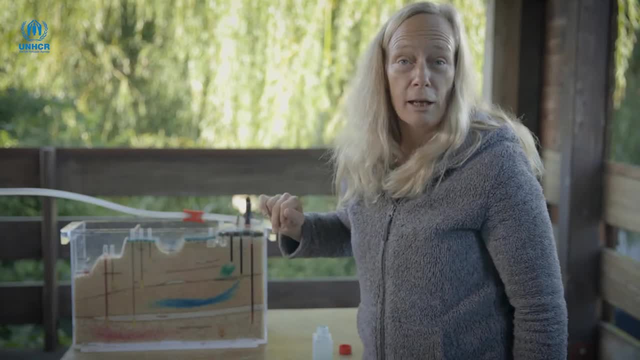 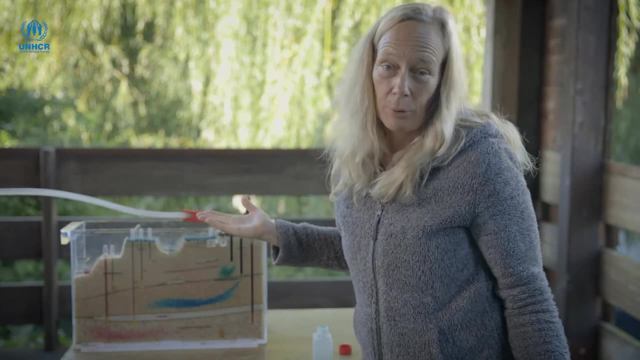 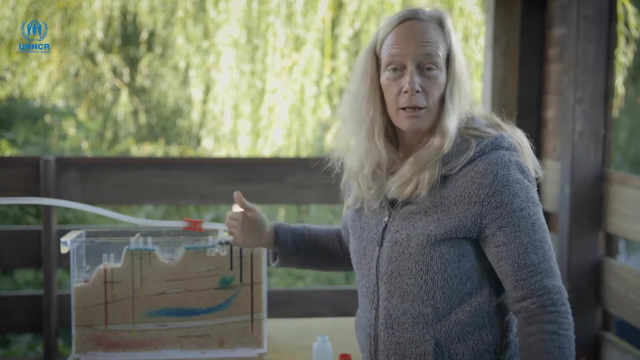 is that you can have two neighbors, one next to the other, and one having a contamination problem and the other one not not understanding what is happening, And this can, in some instances, be. the reason is that the wells are not drilled to the same depth. 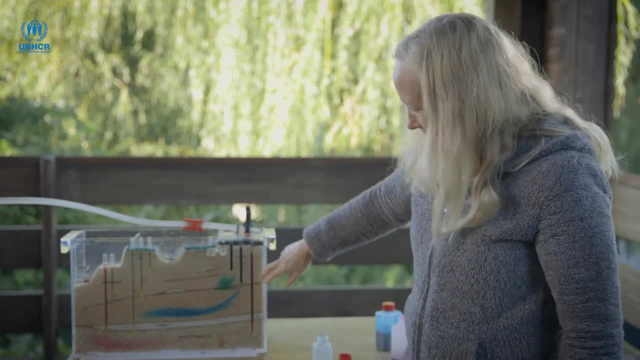 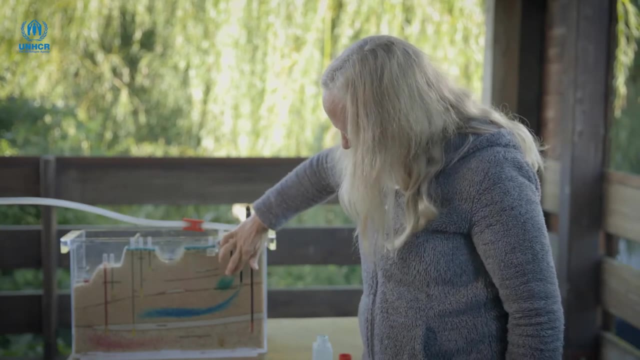 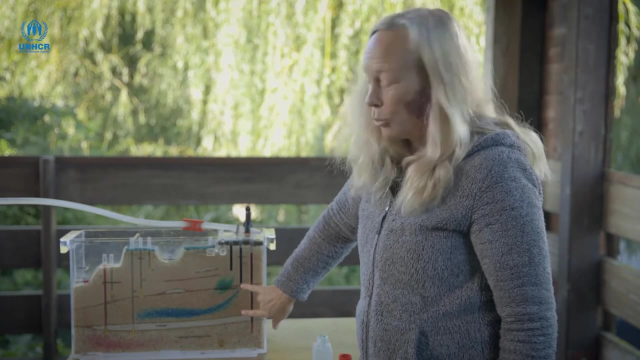 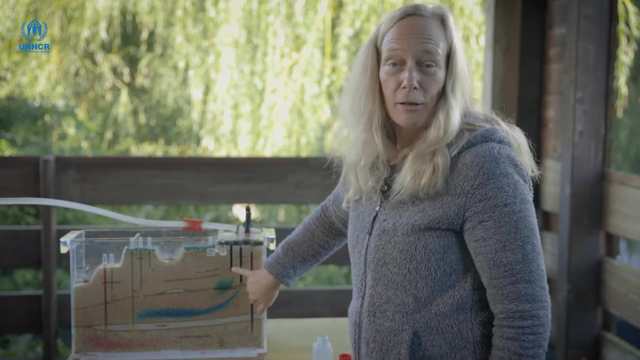 which can explain such phenomena. Now, if you look at this last contamination we've just done, you can see it has gone almost very steeply downwards into this medium-grained layer. Why is that? Well, it is a little bit like with everything tries to take the path of the least resistance. 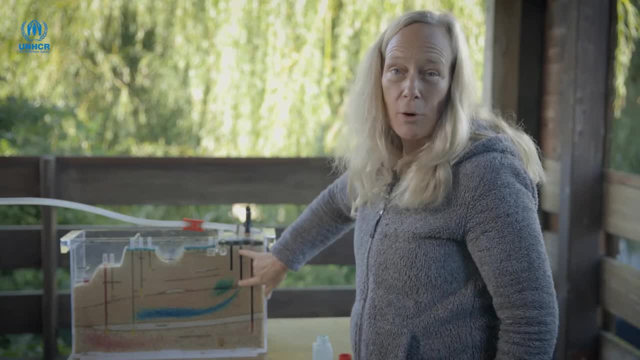 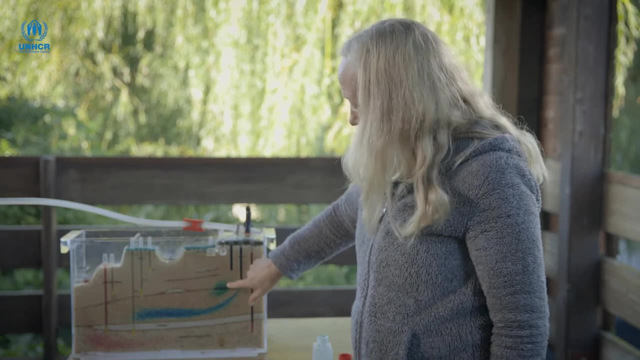 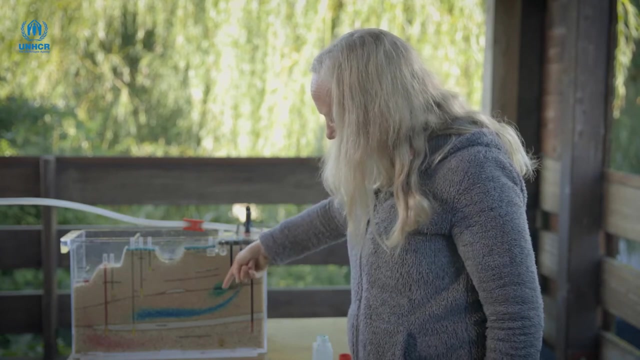 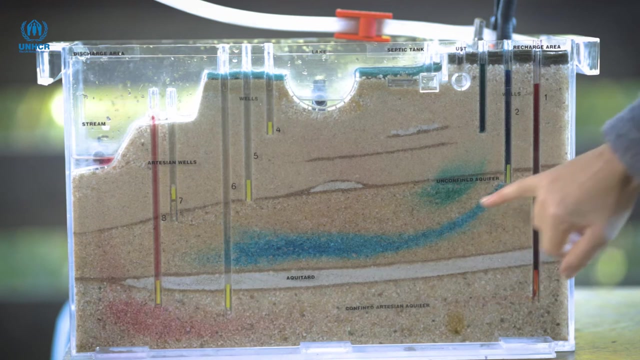 So it is being in this fine-grained material. it is much. there is much more resistance in this fine-grained layer than here. So the pressure distribution forces the water to go down in order then to go along the easier path. Now we can see that this contamination plume here is also starting to arrive. 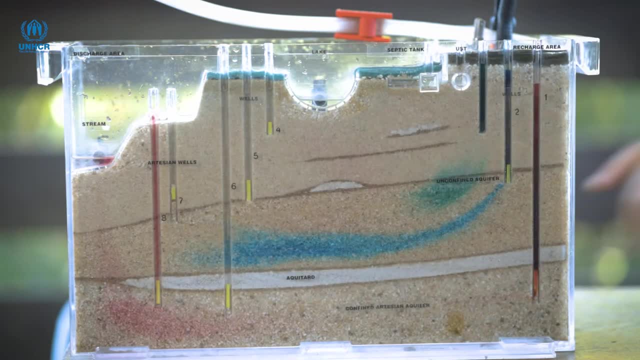 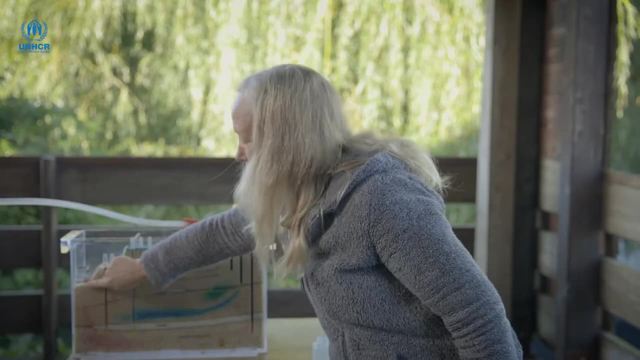 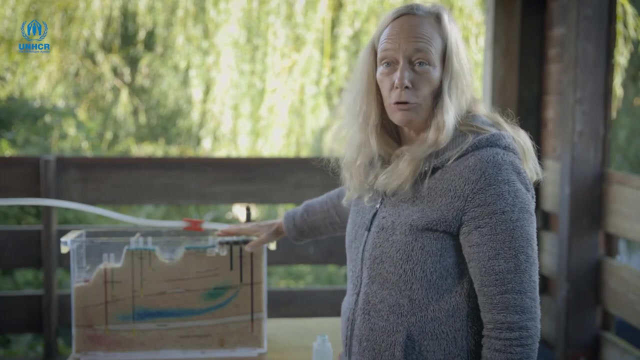 probably also at this neighbor's place, And we can see very nicely now how this red contamination plume is coming up to the stream. So this is an interesting observation that one can make, that you can have a contamination plume. You can have a contamination in a far away remote area. 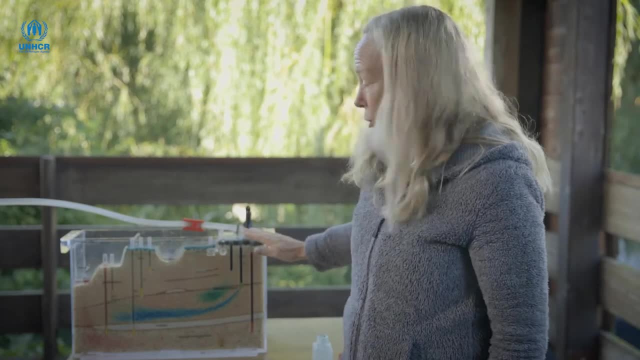 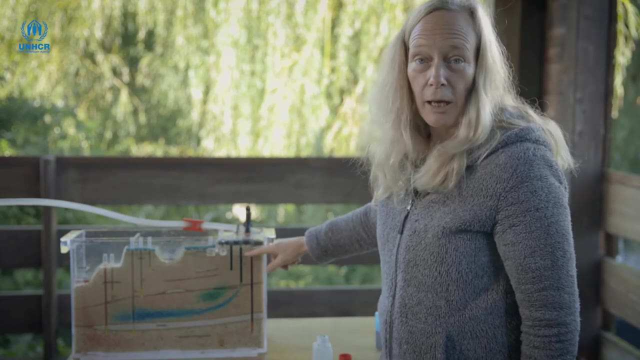 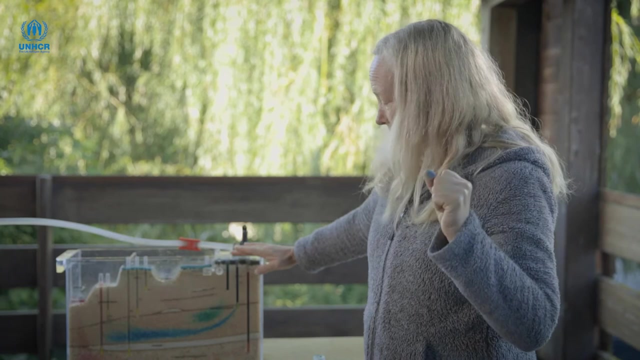 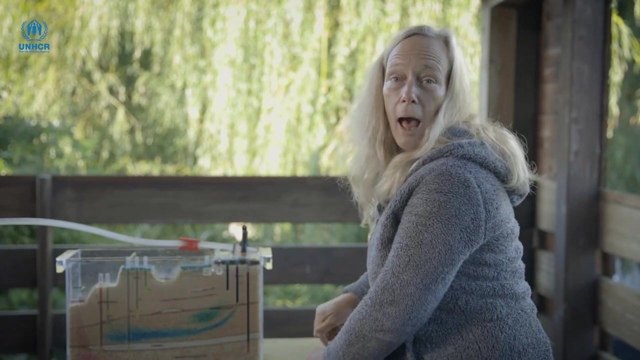 and suddenly you can even get contamination in surface waters or in wells that are far away. So these contaminations that we have looked at just now, this is what we call point contamination. So they are contaminations coming from singular points, What we often have if we are talking about agriculture. 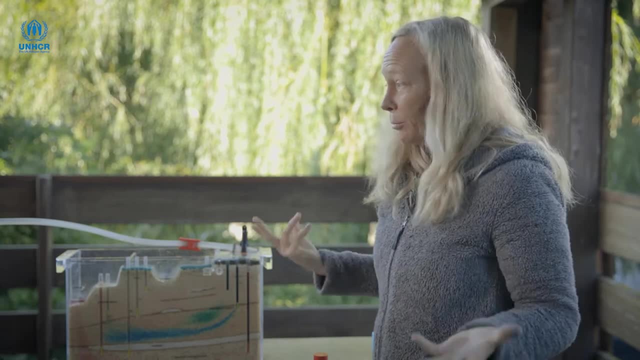 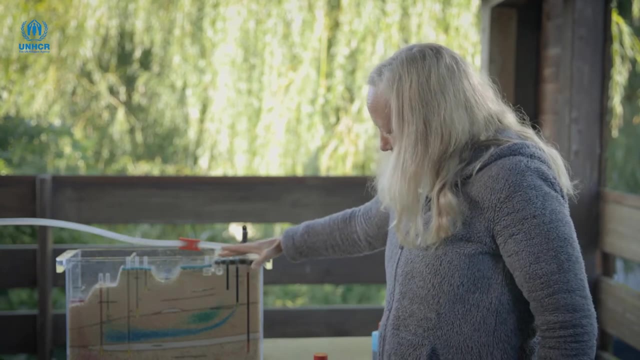 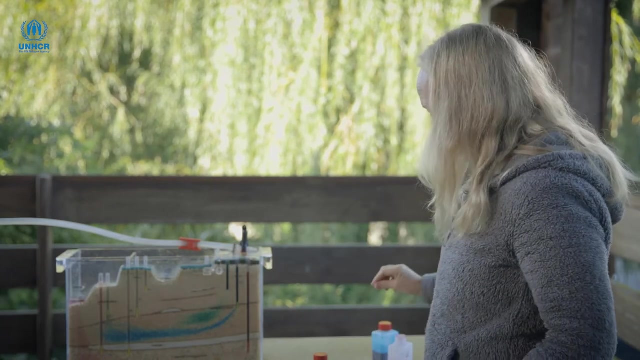 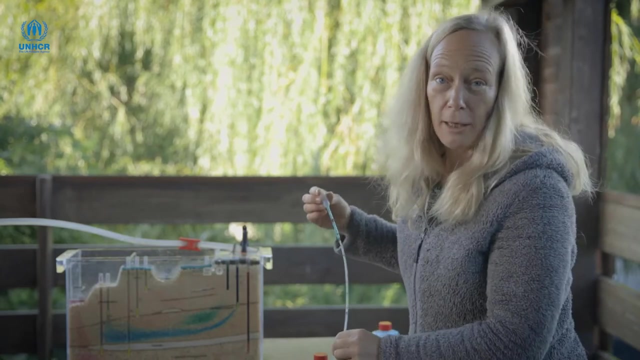 or big areas that are contaminated. then we talk about diffuse contamination. So this would be equal to contaminating or coloring now this whole surface to see what happens. This is now the third experiment we are going to do And for that purpose again, we are going to take the red. 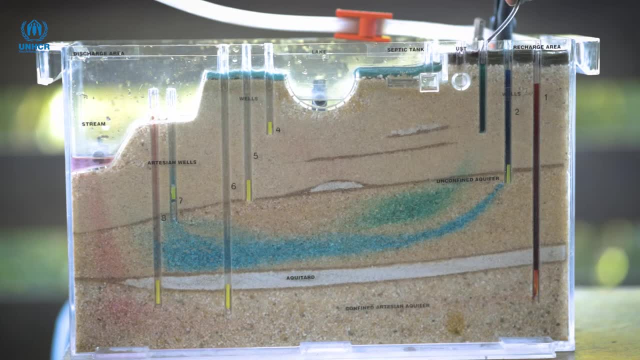 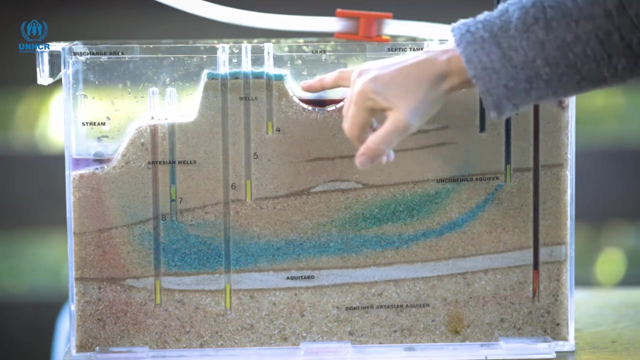 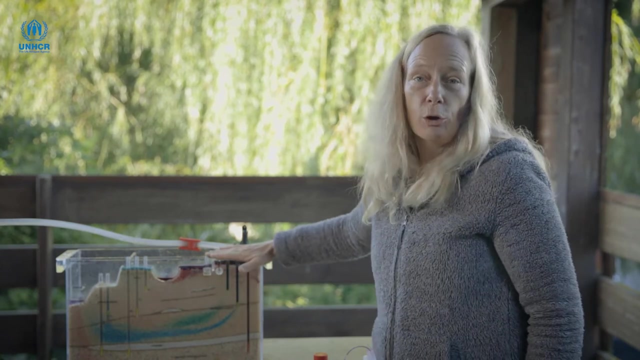 So such contamination can be either agriculture, it can be leaking sewage systems, it can be anything that is over a wide area and you can immediately see the effects. where this whole upper area is getting contaminated, close-up surface waters are contaminated. So that is one of the reasons why one often says: 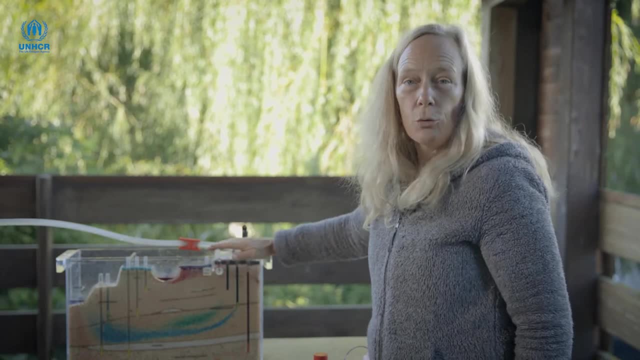 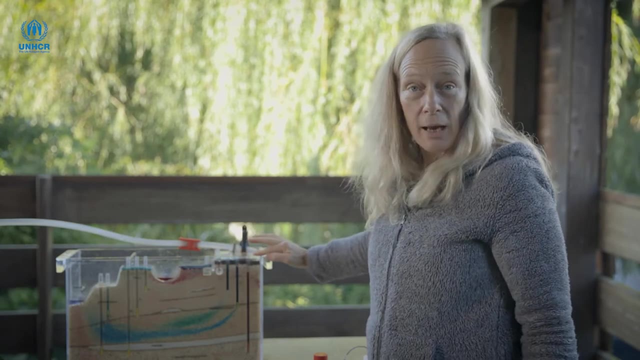 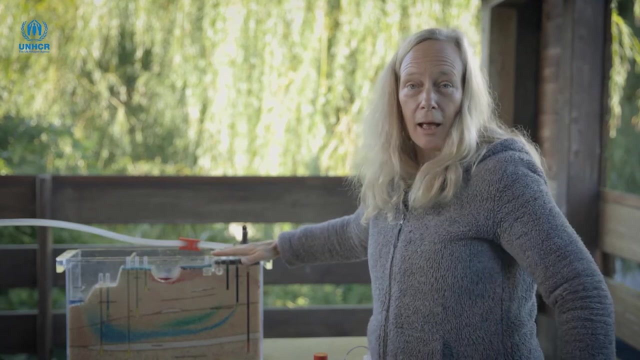 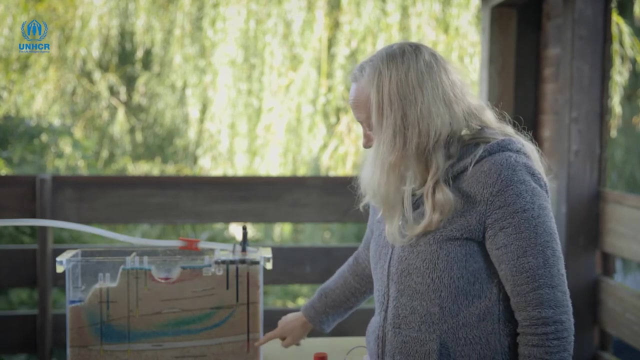 that shallower wells will have a higher probability of being contaminated, because it is very difficult to protect them from this kind of contamination. So in that sense, when one is looking at drilling a water well, one would always like to find an area where one gets some natural protection. 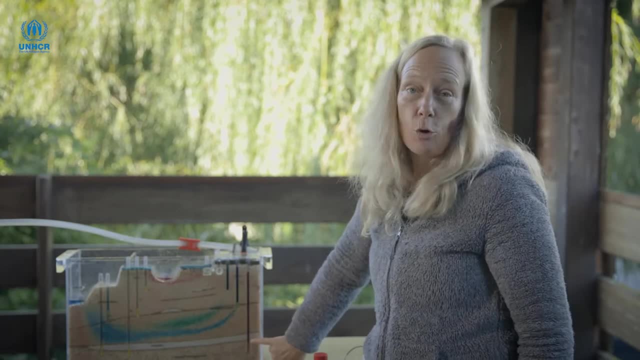 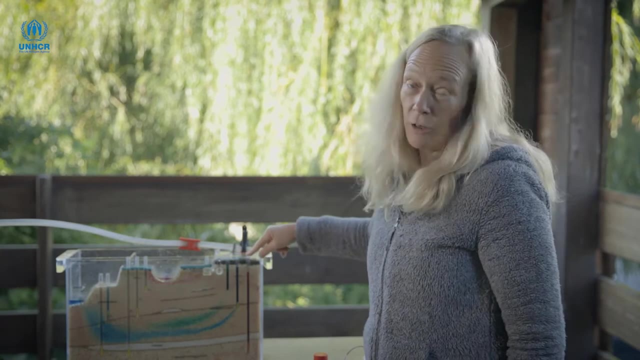 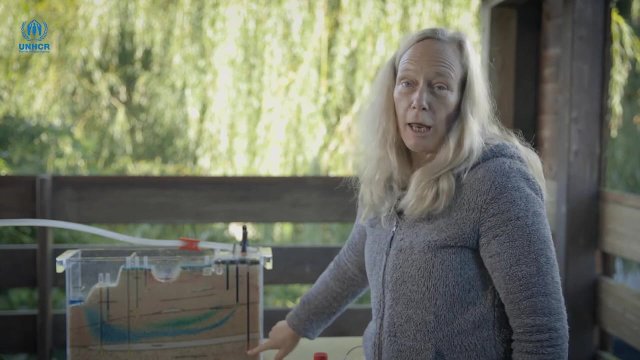 which in this case here would definitely be this lowest aquifer, which is naturally protected by this clay layer. But then again, one has to be very careful. If this well goes into this lower layer, it also means that this well becomes an entry point for contamination. 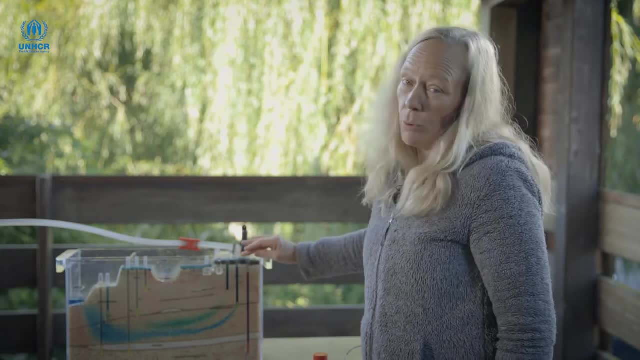 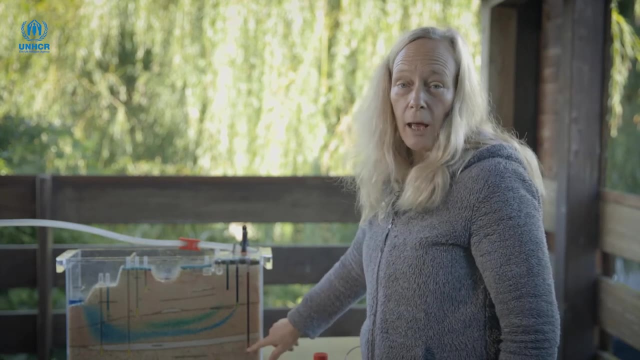 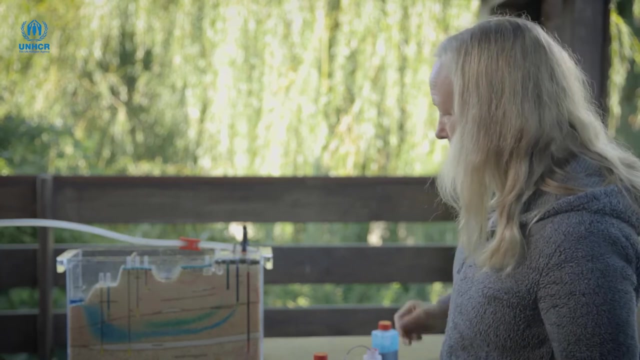 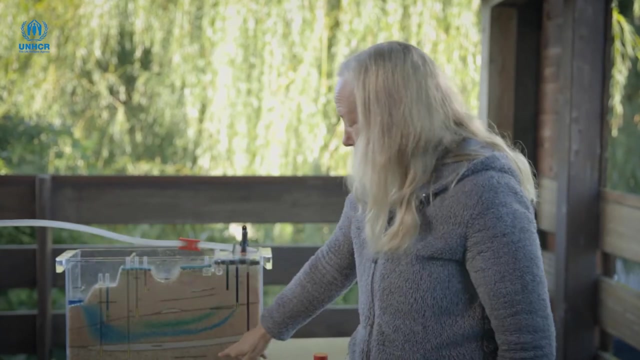 So that is why it is extremely important to make sure that such wells are extremely nicely sealed in order to avoid any sort of cross-contamination along the well itself. So now we can see very nicely that this last well which was contaminated or which was affected by the lowest layer. 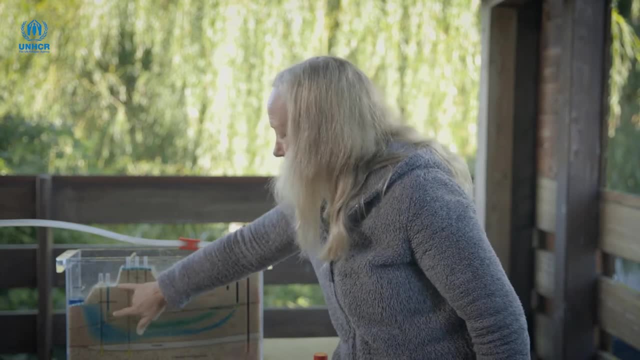 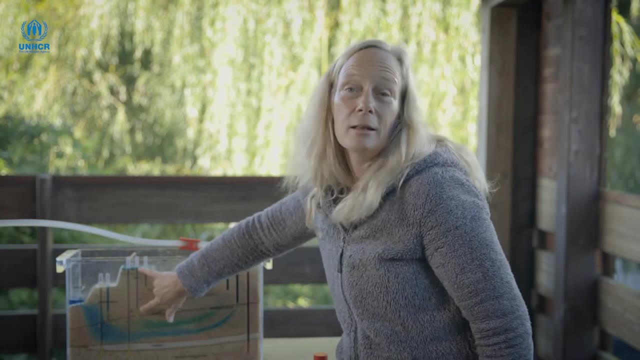 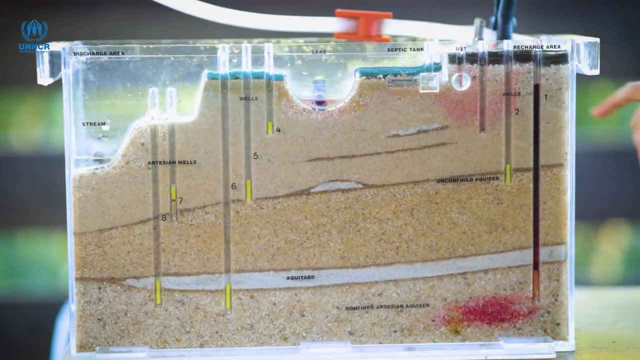 has now a neighboring well which is heavily contaminated by the injection of this second well, And now this well here in the middle is just about to be contaminated by the third. So we can see that the pathways going from one point to the other, 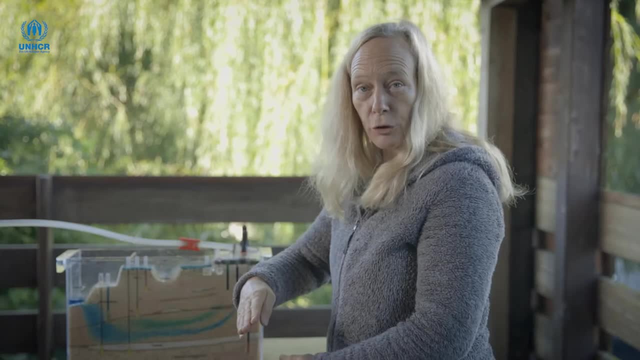 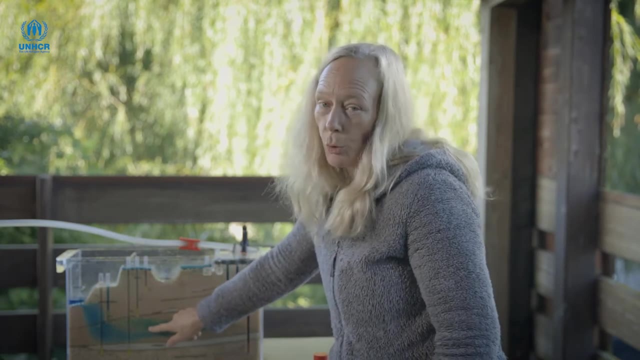 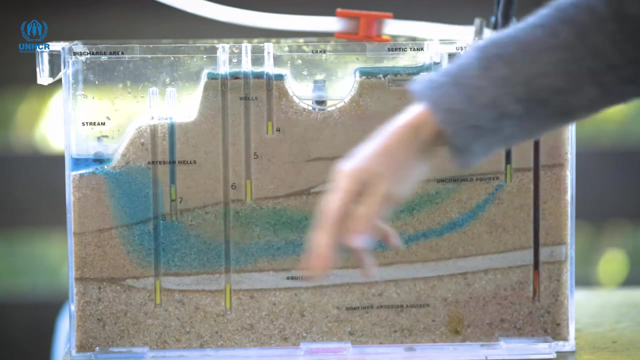 they go to different places and they will never cross each other, but they can mix along the boundaries. So this is also what we call dispersion. And again here it is very nice the movement upwards That one can see So from the piezometric lines. 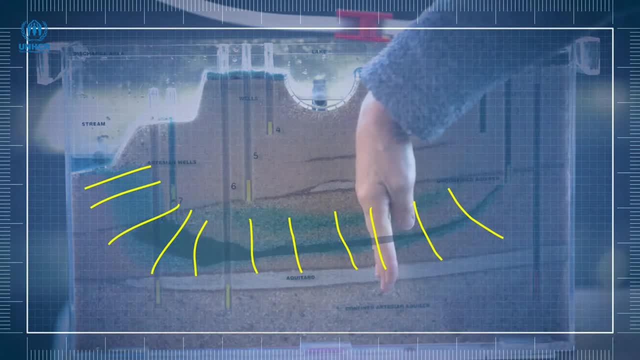 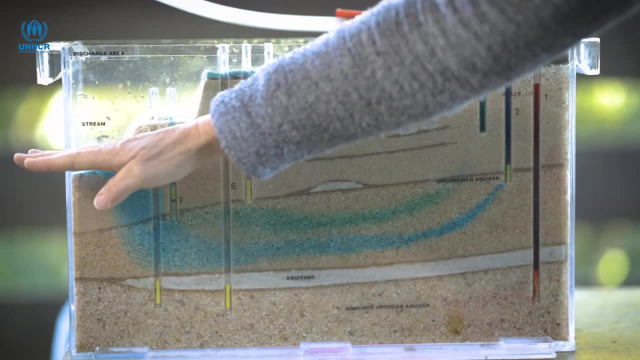 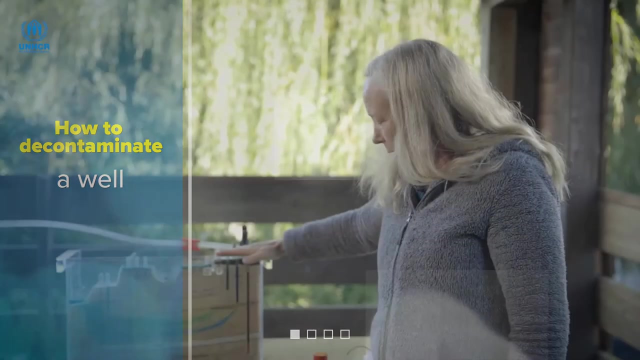 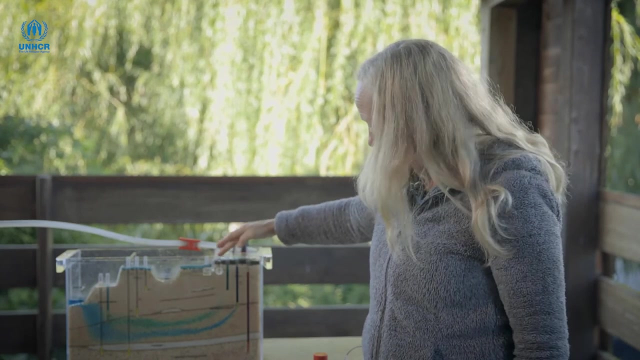 we would see that the piezometric lines are about vertical in this area here, and then bending upwards in this direction. What shall we do? or how can we decontaminate a well once it is contaminated, Because now we have three completely contaminated wells here? 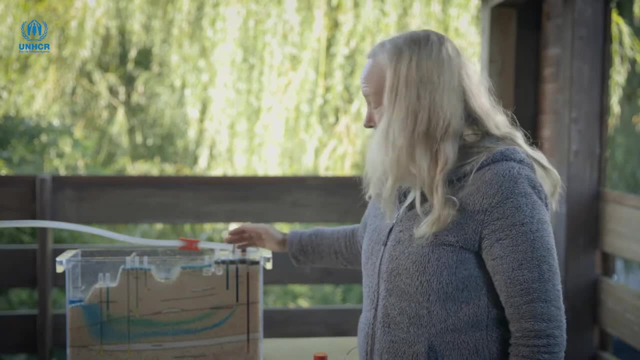 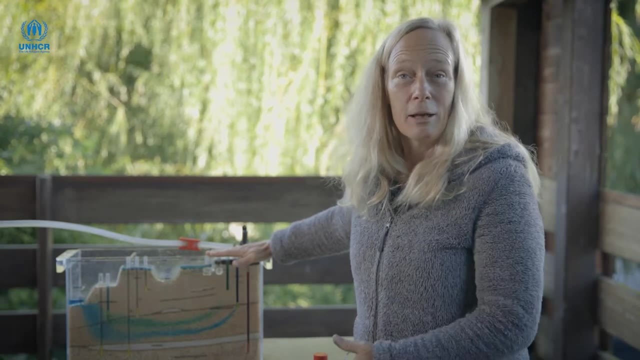 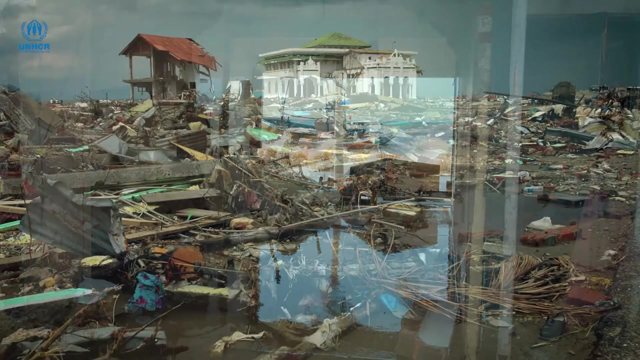 and how do we get them cleaned. So a very nice example for such contamination was, for instance, the 2004 tsunami event, where you have a huge wave coming over massive areas and just injecting sea water into all these wells. So what should one do then? 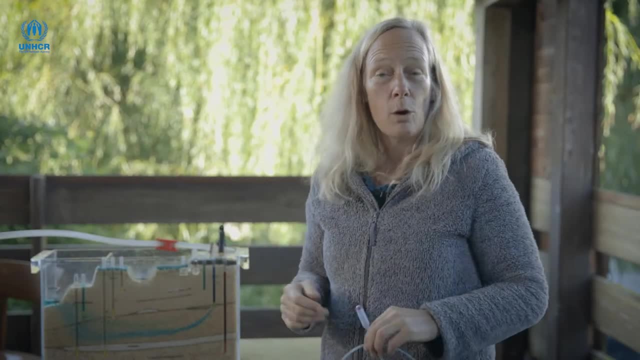 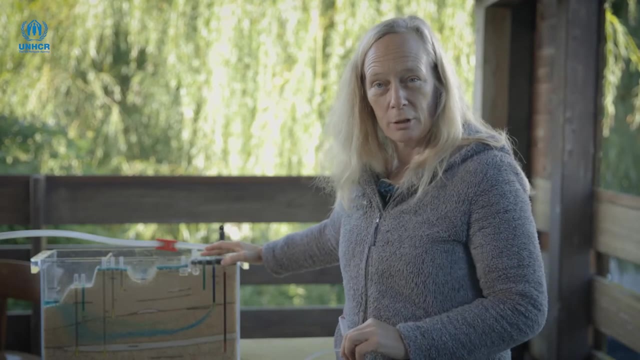 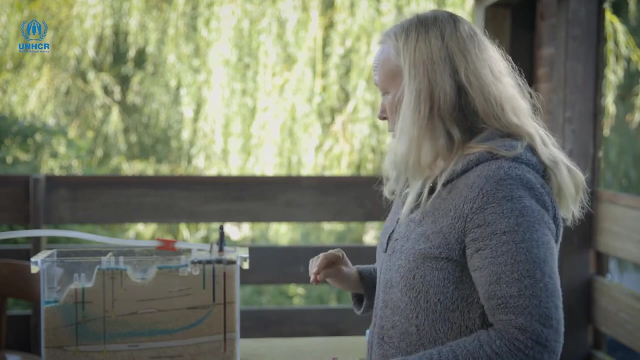 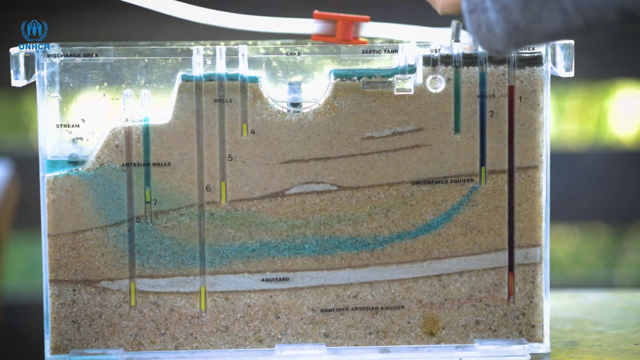 Because, basically, there are two possibilities: One is injecting water into a well and diluting, or the other one is pumping it out. Now, each option has its advantages and its disadvantages. Now, the advantage of pumping out the water is, of course, that we remove the contamination. 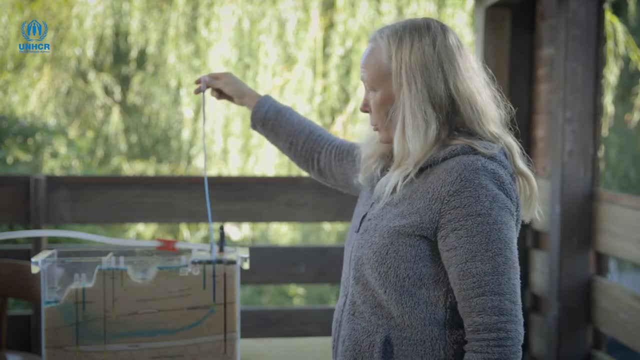 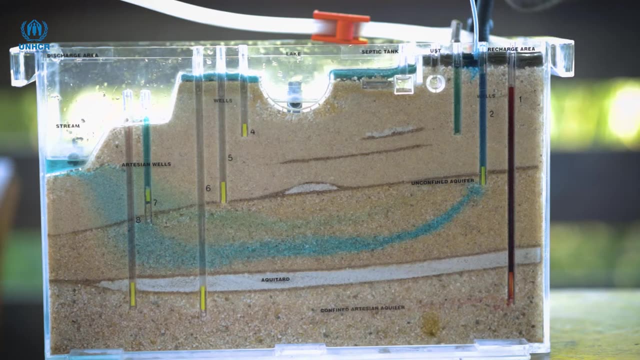 So now I have all my contamination up somewhere, but the very big issue is then not to get rid of it and not to re-inject it just next to the well. So this is one big problem that one may get when one actually pumps contaminated water out of a well. 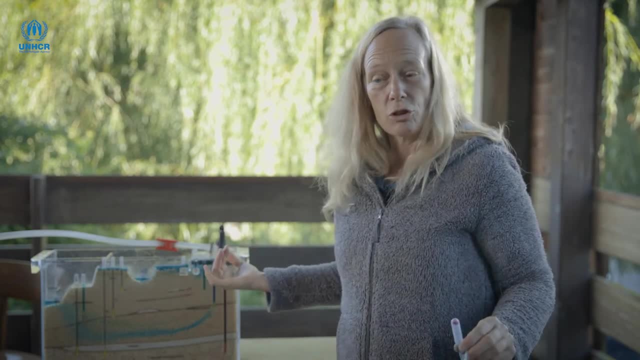 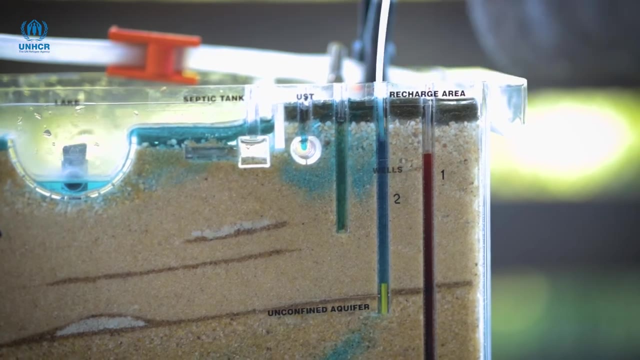 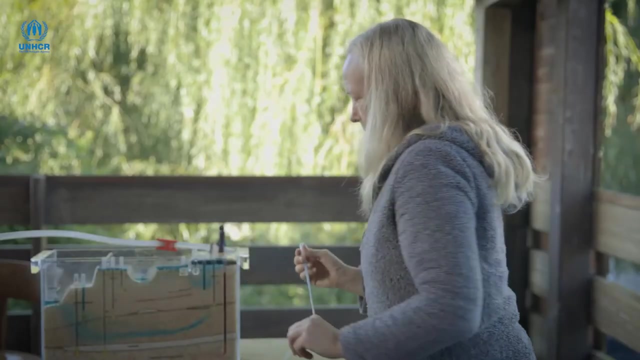 is that one has to make sure where to discharge it in order to get it away and not re-contaminate an area. So this one here we will say: we have contaminated it by pumping. So you can see that by just pumping in here. 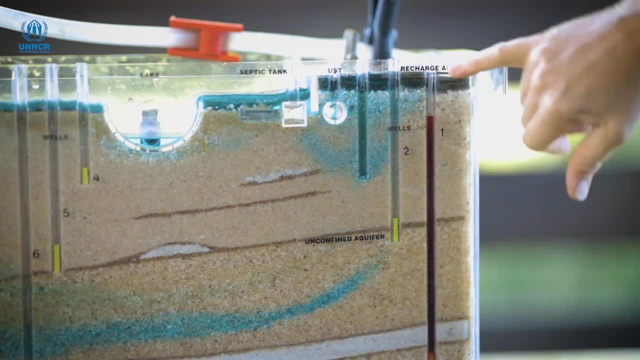 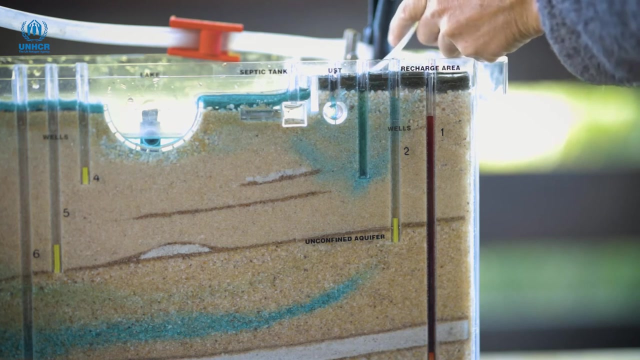 the well has become very clear, but we have introduced the contamination all over. Now the second possibility we have is that we can inject clean water in order to dilute and get rid of it. So this is what I'm doing here. The advantage with this. 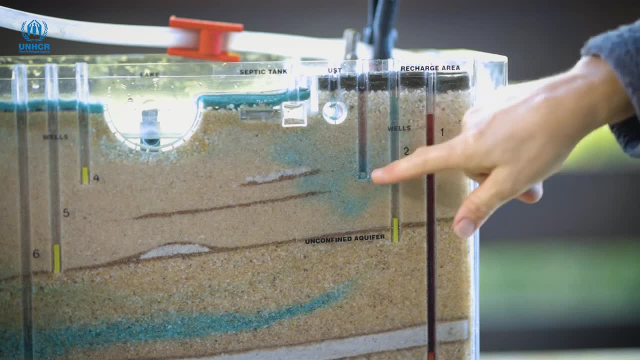 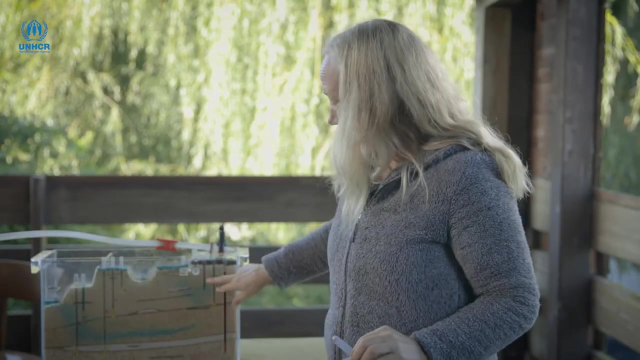 is that you get an effect of dilution. The disadvantage with it is, of course, that you keep your contamination down in the underground and it will just continue its way, And if you don't know where it goes, it will still be there. Now a third option. 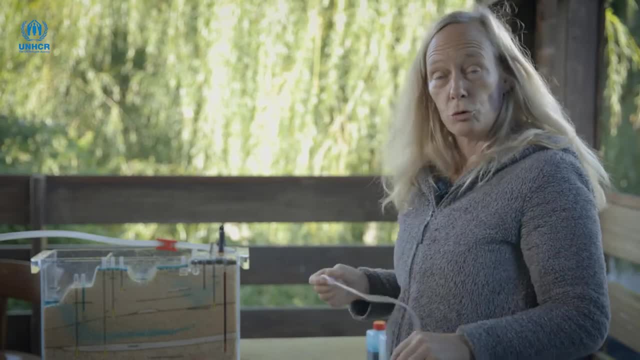 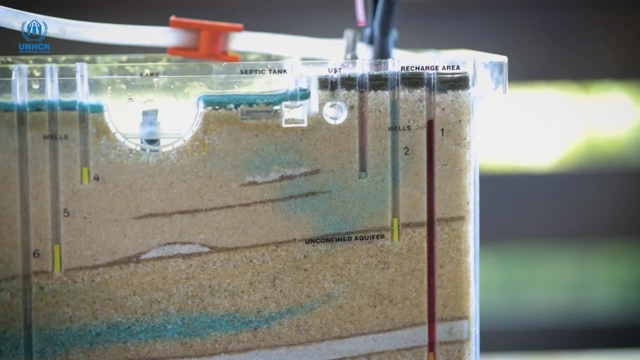 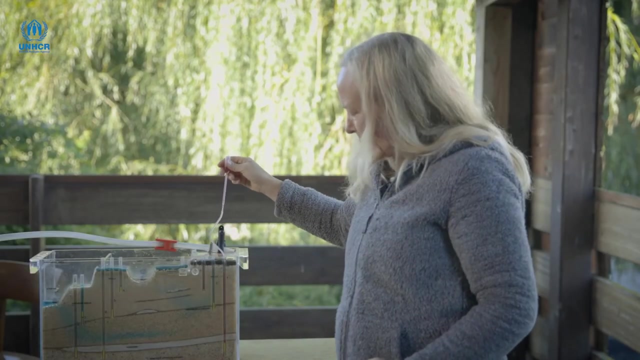 and that can sometimes be a good option as well- is to do a combination of the two, is to pump and to make sure that it is taken somewhere away And then add on it some dilution. in the end, The problem with pumping is that while you pump, you change the water level. So this was one of the things that happened when wells were decontaminated along the seashore is that they pumped so much that eventually they got the water from the sea coming in, causing seawater intrusion. 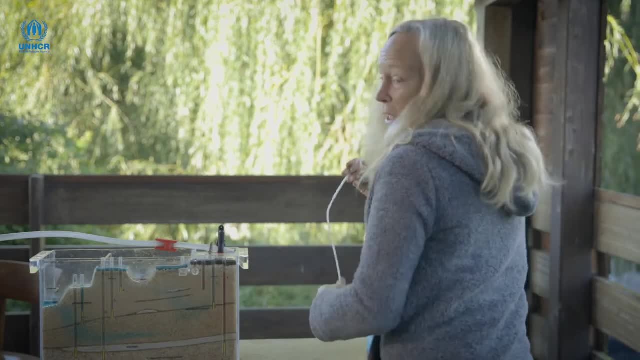 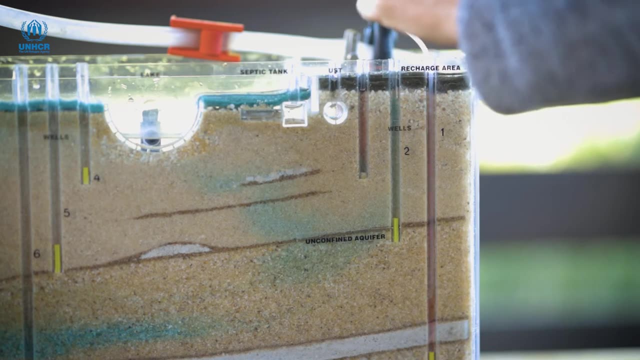 which was a worse contamination actually than what they had in the first place. So in some instances it can be best just to treat and to nicely clean the immediate surroundings of the well and let the dilution of the flow of the water do the rest of the decontamination. 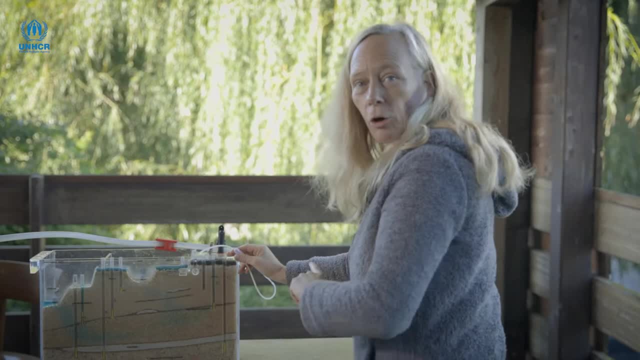 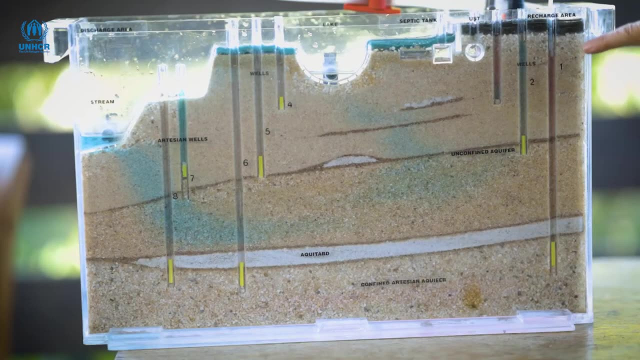 So with respect to effects of pumping onto other wells, here we can have a nice example. If we inject or if we pump in this well which is connected to this well here, if we inject water in this one, you will see that the water is actually coming out. 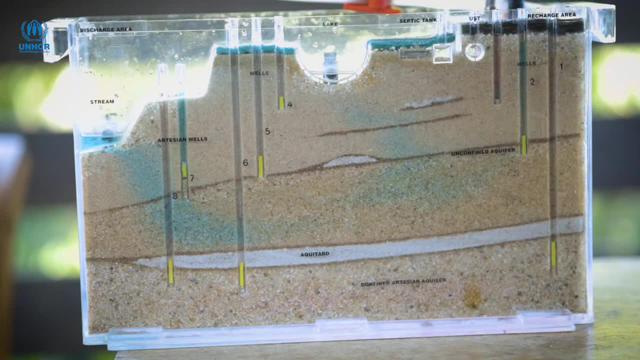 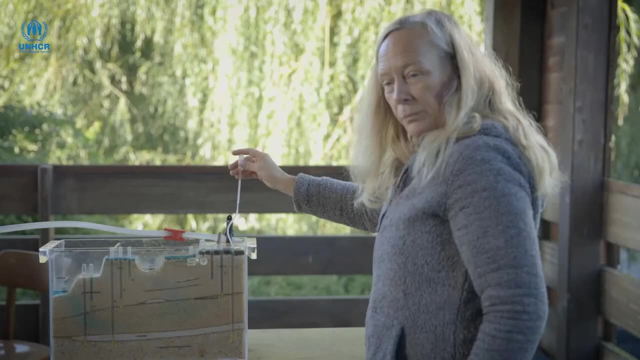 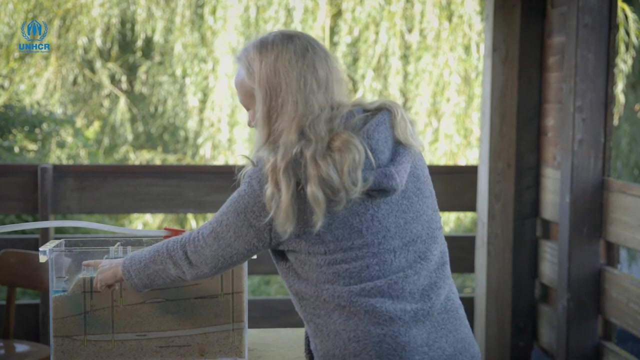 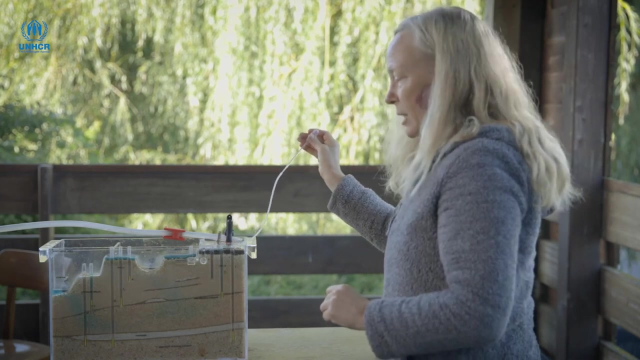 of this one here. Why is that? It is especially in confined activities like aquifers. pressure waves are very fast, are propagated very quickly, So whatever you are doing here will be felt very quickly at the other side. But this is really what you can see. 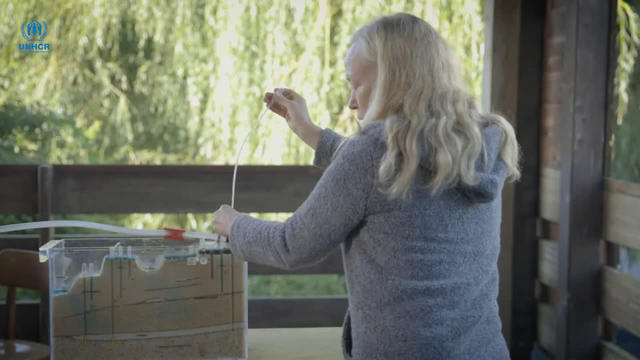 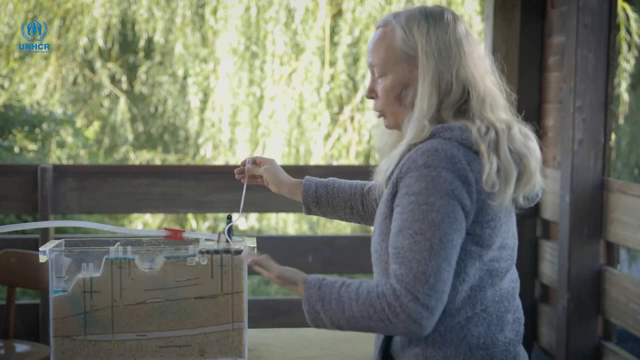 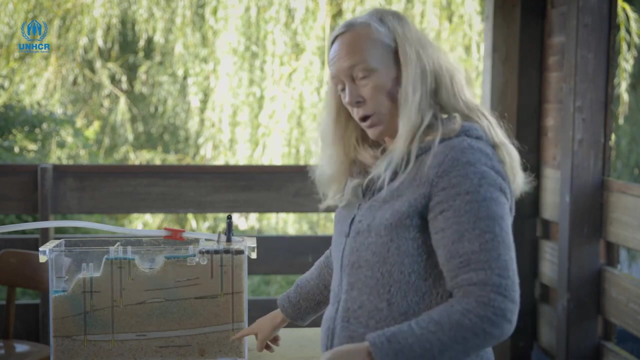 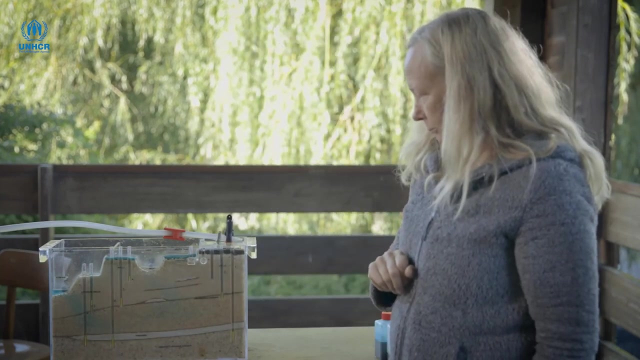 in this area. here, in reaction to the pumping or injecting, is just the propagation of the pressure wave and not the propagation of the molecules themselves, which take much longer time, as you saw before with the propagation of the plume. Our last decontamination is now in the downstream area. 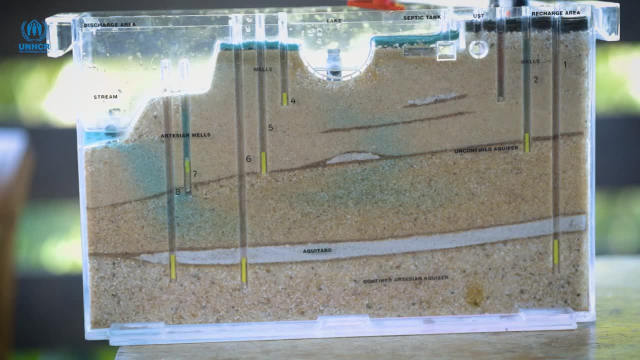 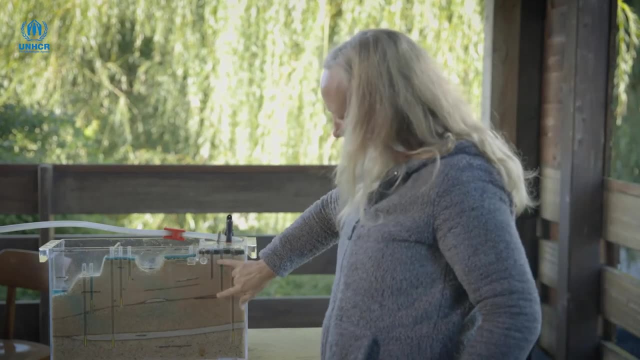 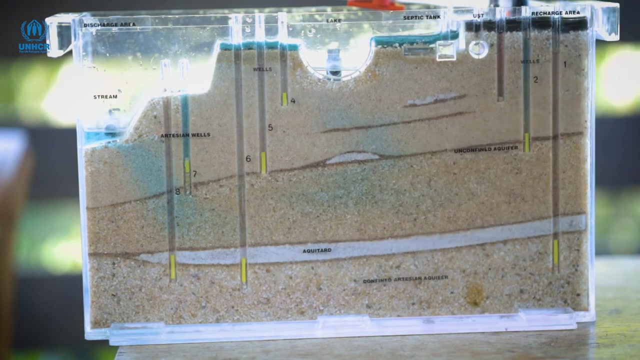 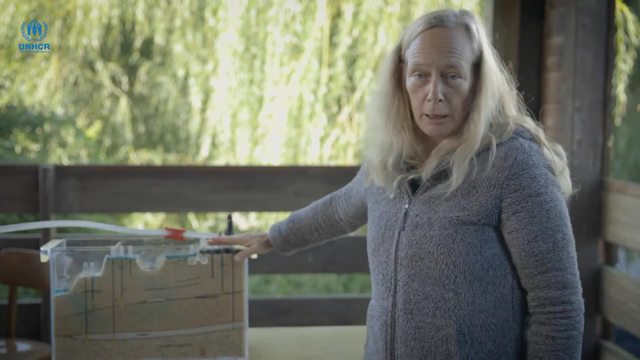 with this. well, here And now it is getting more and more, You can see that the whole contamination in this upper area here is much more diffuse and takes longer time to be evacuated than in this lower part. So this model, basically it allows us to see: